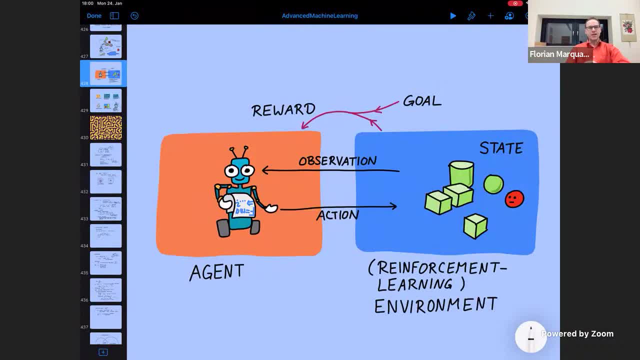 The first item in our list was to deal with words for the different components, Like the agent and the environment, observations and actions, rewards and states, And then we went and discussed two very simple but general schemes for doing reinforcement learning, And the first one was called policy gradient. 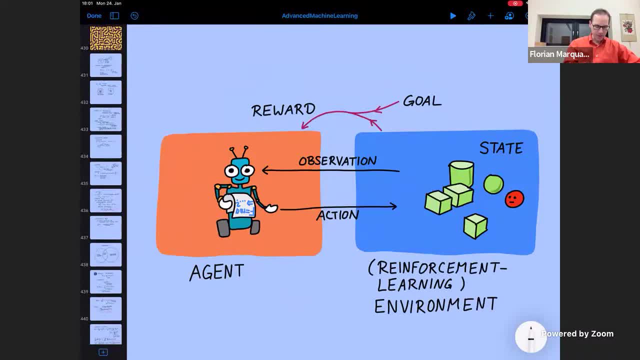 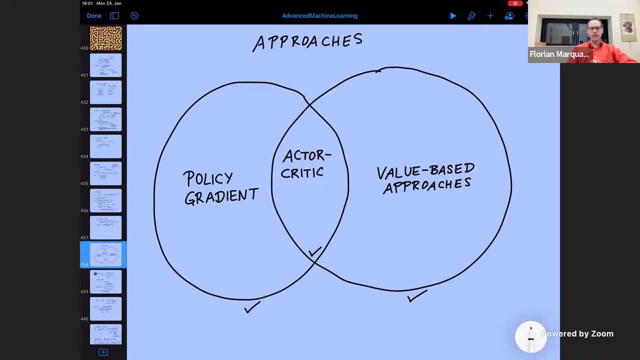 The second one was called Q learning. So to give the bigger picture, which will also become important Today. on the left hand side in this overview we have policy gradient methods that directly try to improve the policy, And on the right hand side we have value based approaches that try to estimate how good is a certain state or how good is a certain action in a state. 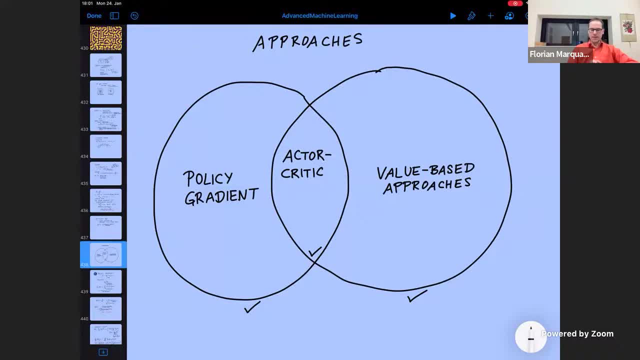 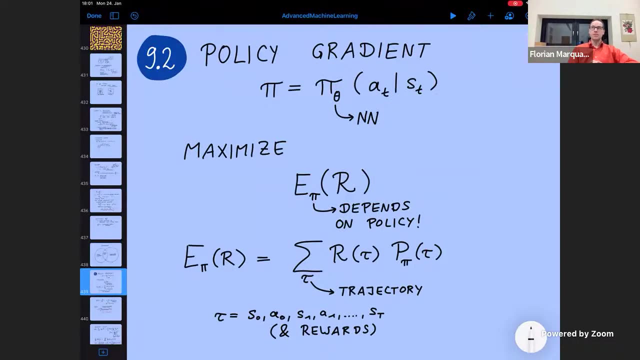 And then from that derive the policy And then in the middle you already see actor critical approaches. This is what we are going to discuss later today, But first as a recap, In policy gradient you imagine that you have a policy that is a probability for taking a certain action given a state. 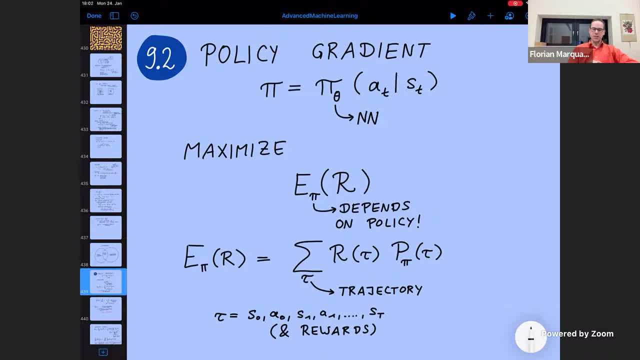 And that this policy would be parametrized with a continuous parameter, theta, for example in a neural network, And then your goal will simply be to do gradient ascent in this parameter with respect to the overall return, to the expected average return, overall trajectories. 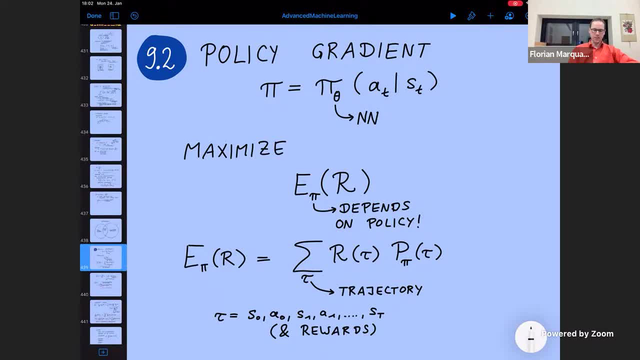 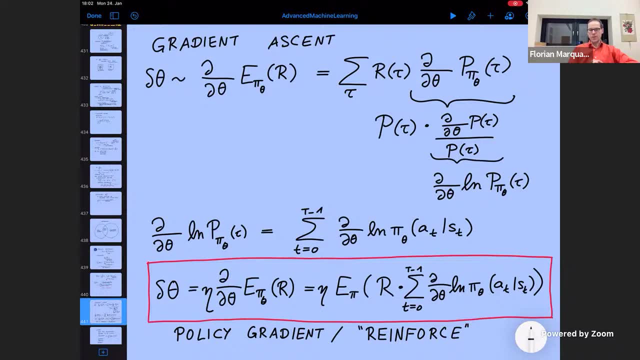 Because that's what you want To optimize. And then, if you go through the math, you find a relatively simple looking formula. Given the generality, it's quite simple looking where the update of the parameters is given by something like the expectation value over all trajectories. 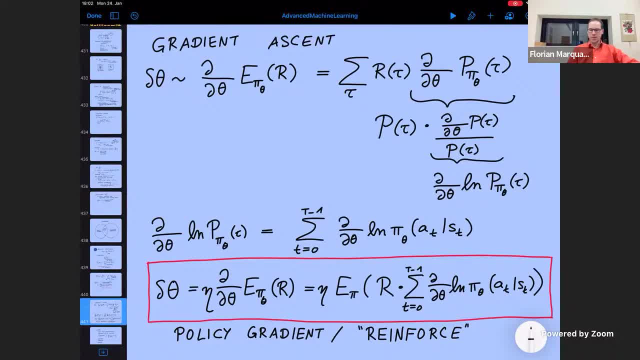 And then the product of the return of the particular trajectory, multiplied with something like the gradient of the log of the action probabilities, and so this is the famous policy gradient formula, and, if you have already started doing the homework, this is what we are applying in this notebook that i put up on the 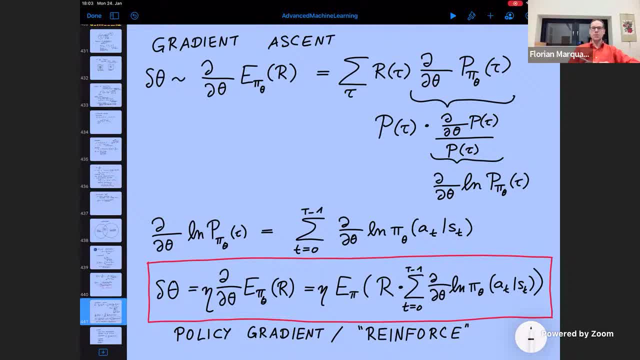 website where you can see how this works in practice if you implement the policy in terms of a neural network and otherwise have a relatively simple states and actions. in this case, it was an example taken from physics where the states were quantum states of a simple two-level. 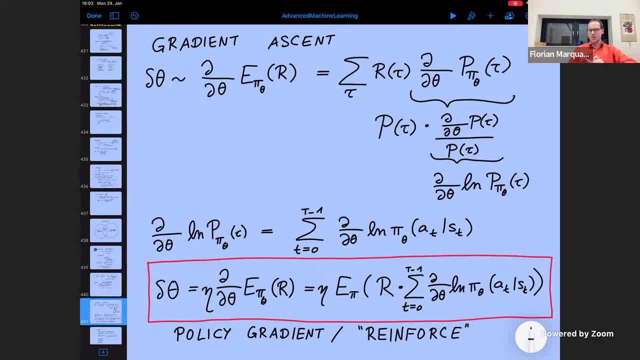 system represented simply as vectors, and the actions were rotations of these vectors, and so you have to select the right sequence of rotations in order to rotate the given vector into some desired direction, and if you are very good at that, then the return will be large. so this is what happens, in that 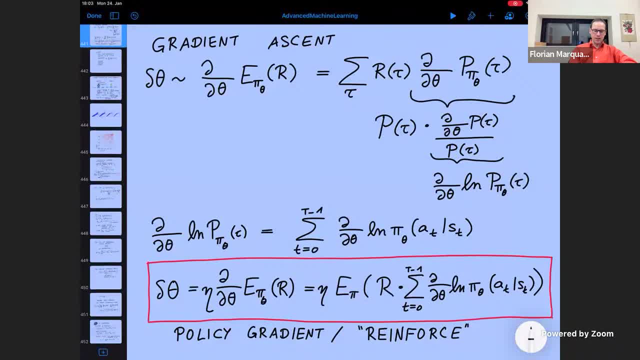 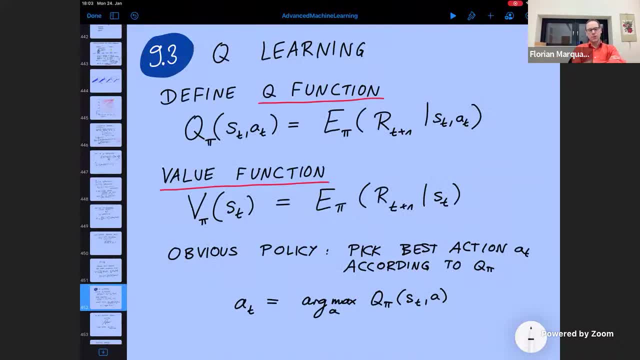 example. now, the next method we discussed after policy gradient was q learning. so q learning is the value-based approach to reinforcement learning and it rests on the q function. the q function tells us simply if i am in a given state and suppose i take a given action. so, for example, i'm at a certain location in a maze. 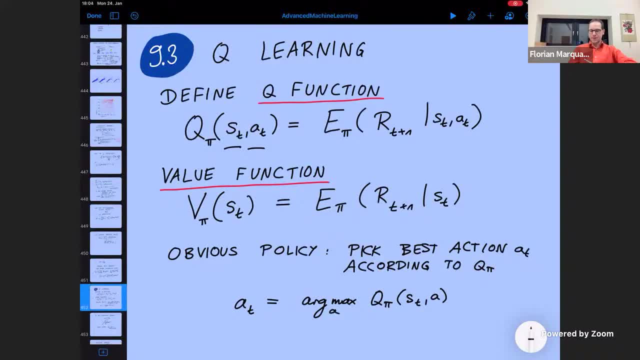 and i move to the left. then, under this condition, what's the expected future return counted from that point onward, the sum of all rewards counted from that point onward? and the obvious policy here would be to say: well, i'm interested in the particular action of course that will maximize the future return on average. 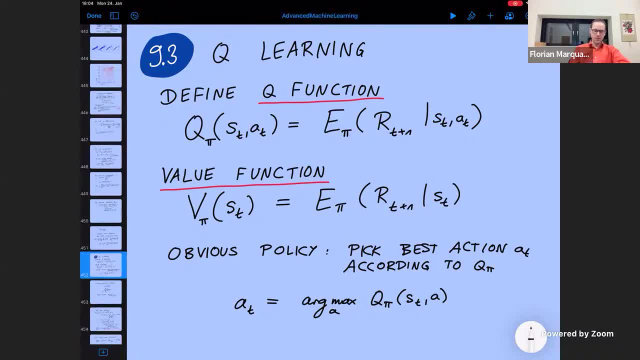 and indeed this will be the action that you choose. so the problem with that is, these expectation values do depend on your policy and the policy in turn depends on the q function. so what you hope for is that you can make this converge towards a self-consistent solution, which 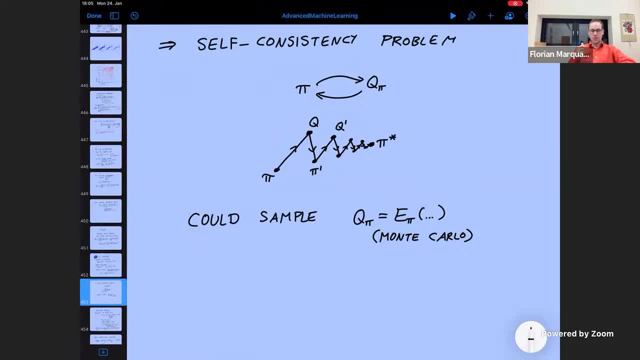 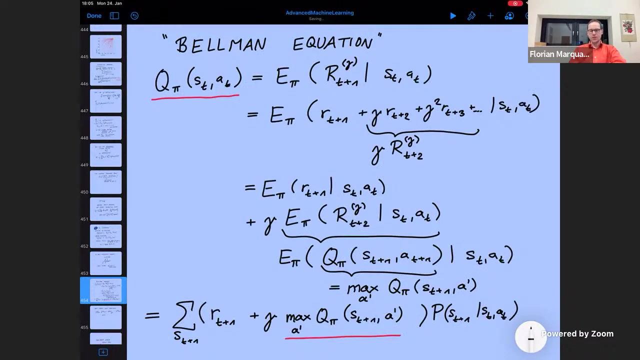 is the optimal policy, which is related to the corresponding q function, and then, if you ask for the best action in this corresponding q function, you always select the action that you would have selected anyway according to this best policy. so they are consistent with each other. okay, and then the question is: how do you figure out what is the q function? 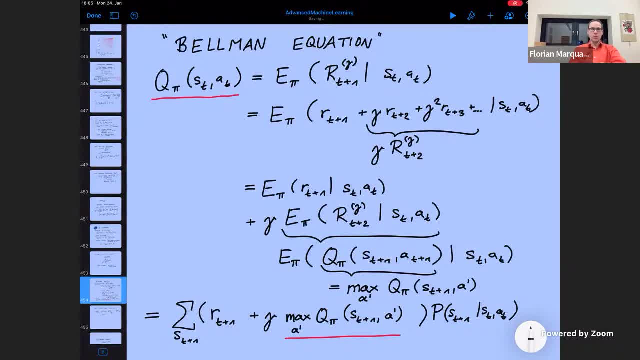 and you could literally do, so to speak, monte carlo, in the sense that you start in a central state, take a certain action and then you run stochastically many trajectories, record the returns and take the average. so that would define the q function, but it may be expensive. 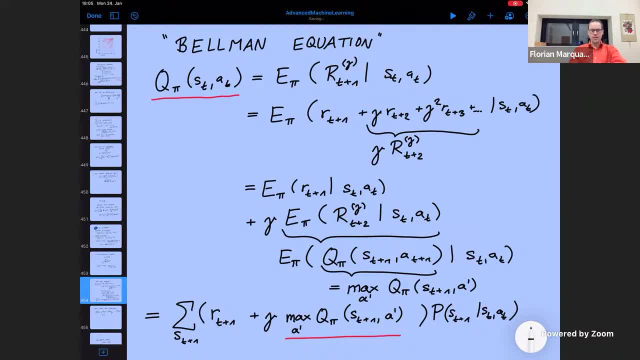 so what people have come up with is a self-consistency equation that essentially says the q function at some state and for some action is the return that i would get from the state and action in the next time step, plus all the rest of the return, and that again can be expressed in terms of the q function. 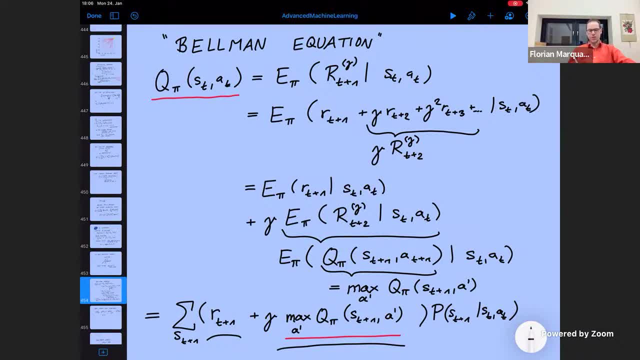 namely maximizing over the next action, because that's what our preferred policy and q learning would tell us to do, and the q function here represents the rest of the return in all future time steps, and so this is obviously a self-consistency equation. so the q function 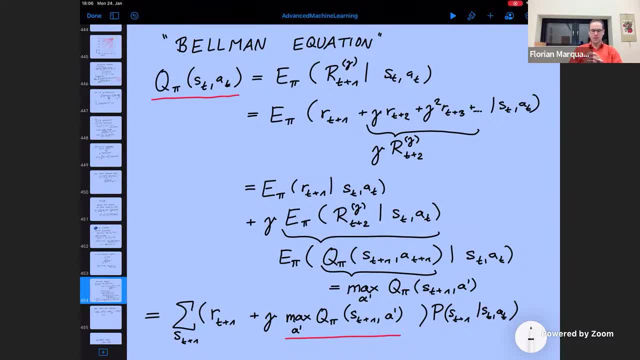 appears both on the left and right left hand side and on the right hand side. and the way to solve such an equation- at least one way to try to solve it- is to start with a guess for the q function and then always use this guess on the right hand side to obtain some new guess for the q function that is on the left hand side. 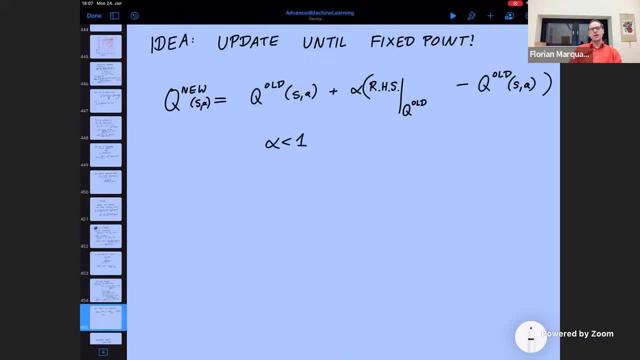 and then to iterate. so you have a fixed point iteration and when nothing changes anymore. so the new q function, predicted by the bellman equation, by the self-consistency equation, is the same as the old one you already had. then you have a reached convergence and then that defines. 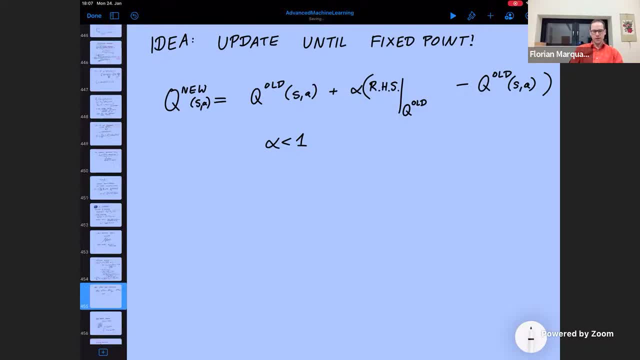 your q function okay. so we said how this works in principle. in such a fixed point iteration you would take the difference between whatever is on the right hand side of this self-consistency equation and the old q function. if the difference is zero, that means you have converged, but if it's not zero, then you multiply. 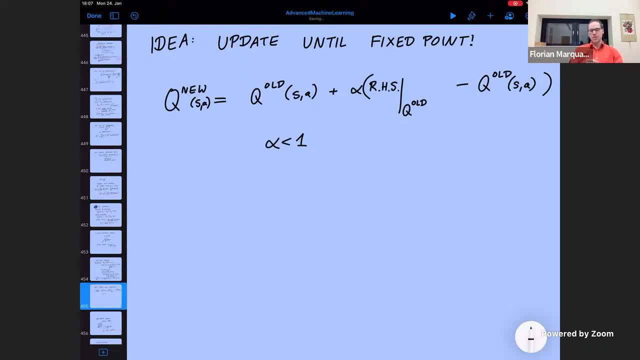 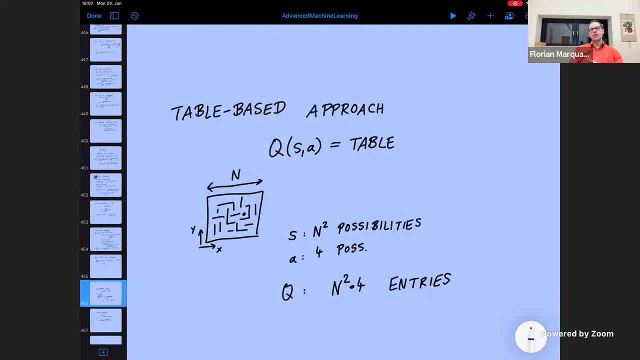 that with some number, alpha, that is, so to speak, the step size, and you add it to the old q function and that tells you what is the new q function. so you take a little step in the right direction. and last time we saw how this works in practice. if you have an example, in this case it was a maze. 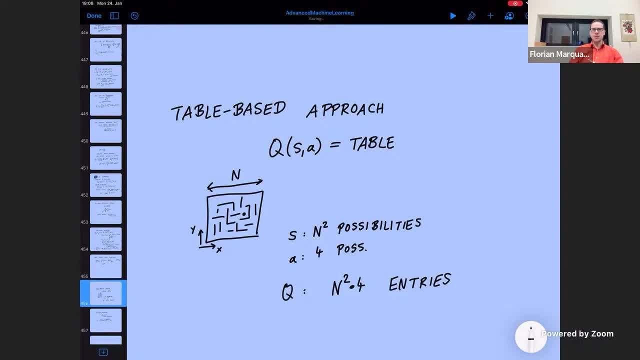 where the number of states and the number of actions is still relatively small. if the numbers of states and actions are relatively small, then you can simply make a table so you can store the whole q values inside a big table and update it according to this equation: iterate until it. 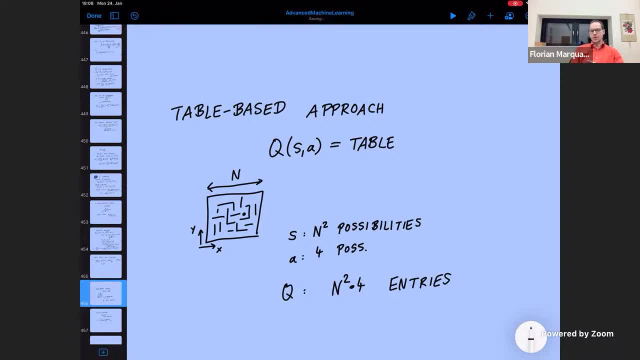 no longer changes, and then you have your q function for the optimal policy. but sometimes this doesn't work. sometimes the state space or the action space is simply too large, and then of course the answer, as you can guess, is try to approximate the q function somehow, and our preferred method of approximation- for any 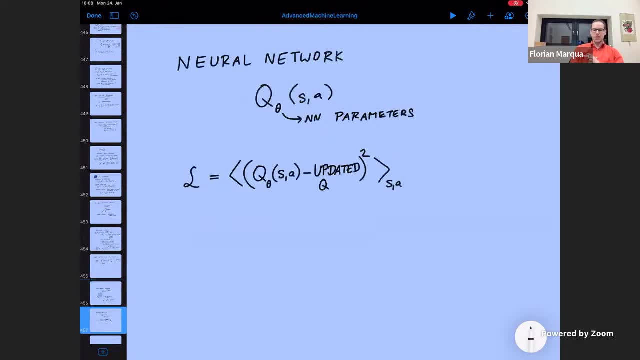 function on neural networks. so you would take a deep neural network where the input could be the state and the action and then the output of that neural network would be the q function. and then you would try to get close with that neural network to whatever your bellman equation tells you should be the 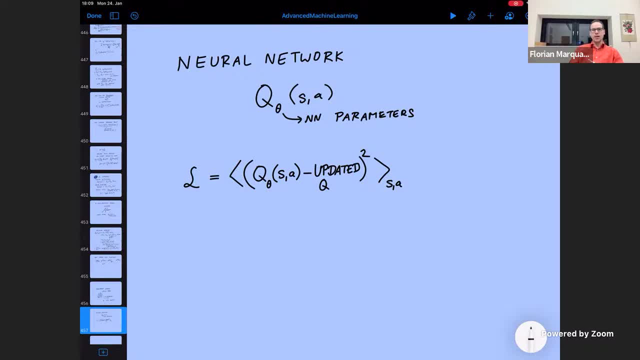 new value of the q function. maybe you can take the mean square error between the two quantities as usual and take that as your loss function and train the neural network to get closer to what the bellman equation wants it to be. now here's a slight little first comment. sometimes it's also 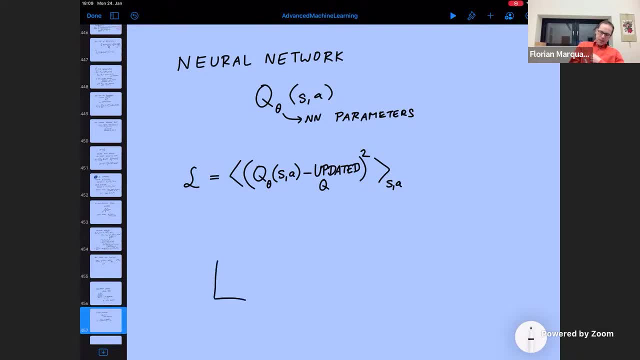 good if, instead of having the, the state and the action as input to the neural network and the q function as output, you have, so to speak, you have another neural network in which only the state is the input, but you only have a selected small number of discrete actions, and then you can have simply several neurons as output and they represent the q function for the different action values. so, for example, there might be a number of discrete actions and then you can have simply several neurons as output and they represent the q function for the different action values. so, for example, there might be a number of discrete actions and then you can have simply several neurons as output and they represent the q function for the different action values. so, for example, there might be a number of discrete actions and then you can have simply several neurons as output and they represent the q function for the different action values. so, for example, there might be a number of discrete actions and then you can have simply several neurons as output and they represent the q function for the different action values. so, for example, there might be a number of discrete actions and then you can have simply several neurons as output and they represent the q. 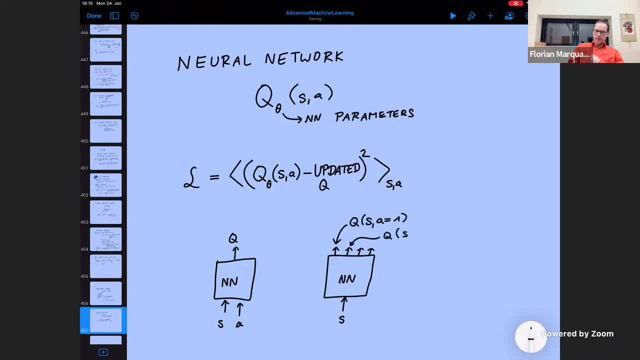 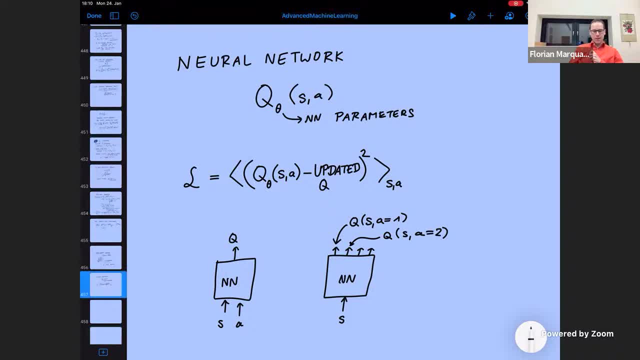 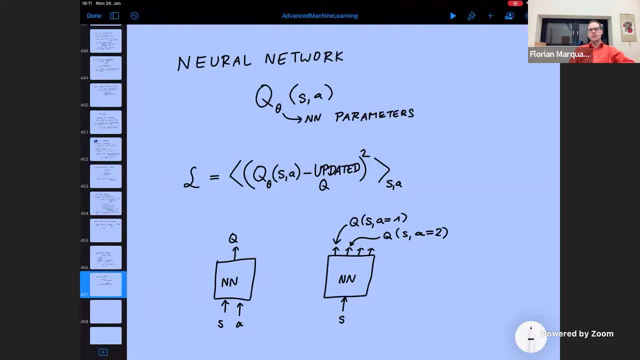 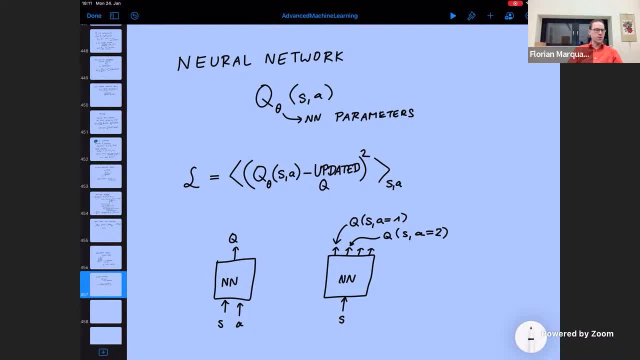 function for the different action values. so, for example, there might be a number of discrete actions and then you can have simply several neurons as output and they represent the q. certain actions are really, let's say, zero or very, very tiny. then also you wouldn't. 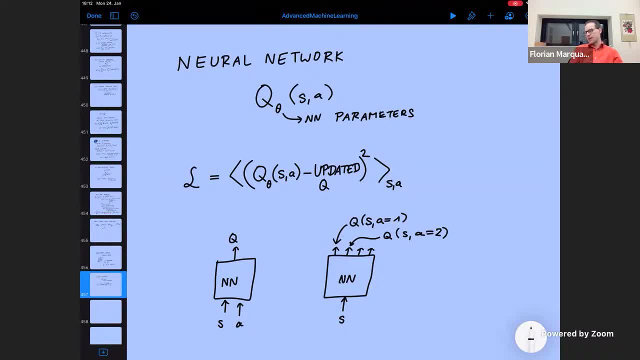 find an update from that, Then, more practically speaking, you can ask: okay, what happens if the best policy requires a very long sequence of very precise actions, and only this one sequence of actions will give you a high reward, a high return, and every other sequence of actions will give. 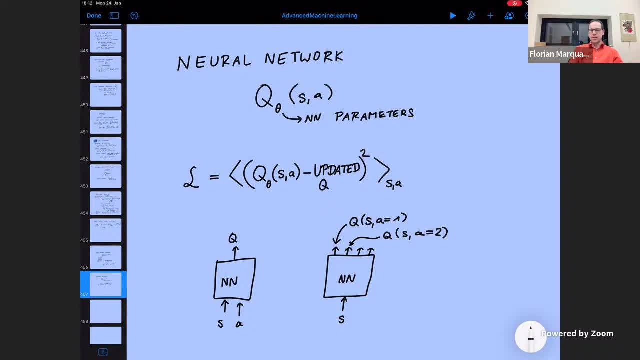 you zero return. That's a particularly bad example. So that's almost impossible that reinforcement learning will work, And that's true both for Q-learning and policy gradient, And the reason is simply that it's so very unlikely to hit this particular sequence. 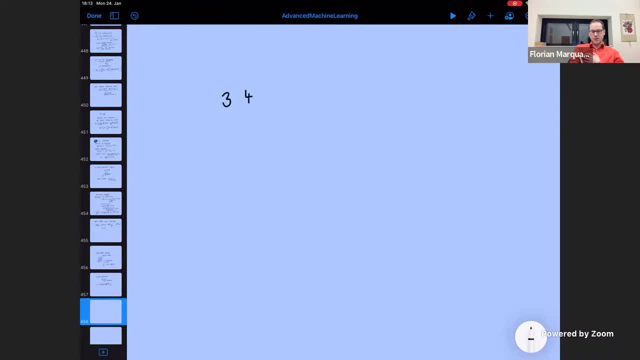 because it's basically, It's basically like a combination. look, So let's say you want to find this particular combination and only then you get rewarded. And then, of course, here there are one, two, three, four, five, six, seven digits. 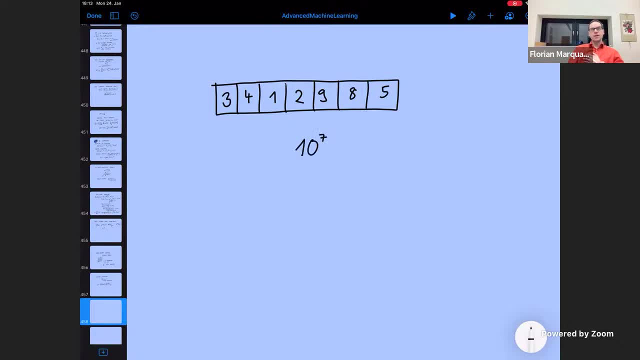 That means there are 10 to the seven combinations, And so if only one of them, So this is a bad scenario for RL. If only one of them gives you a return of, say, one and the rest gives zero, then if 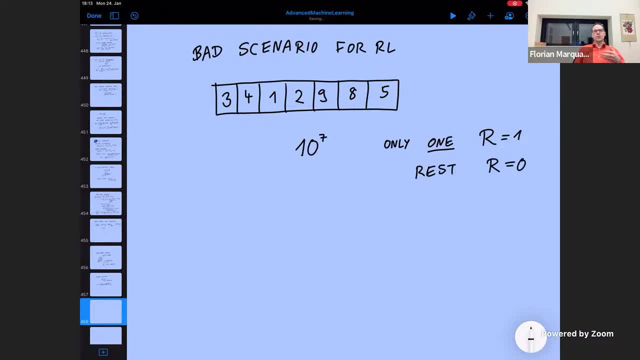 you think about it, in brute force search you expect on average to have to try well, one half of 10 to the seven configurations on average. And actually Okay, I think both policy gradient and Q-learning will not really be better than that, because 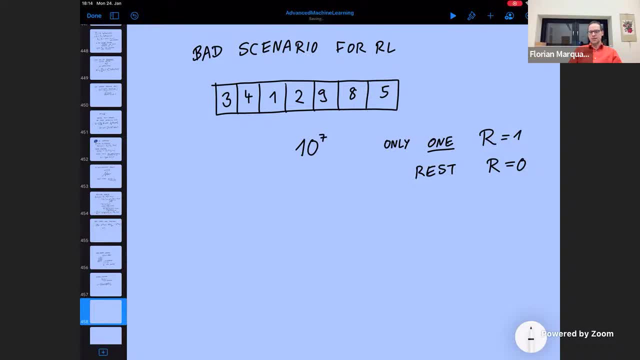 in policy gradient, to get any interesting update, you need to hit the good sequence at least once, And likewise in Q-learning: if you never hit on the sequence, you can never get an update for a Q value that is non-zero, And so also you will never converge to anything. 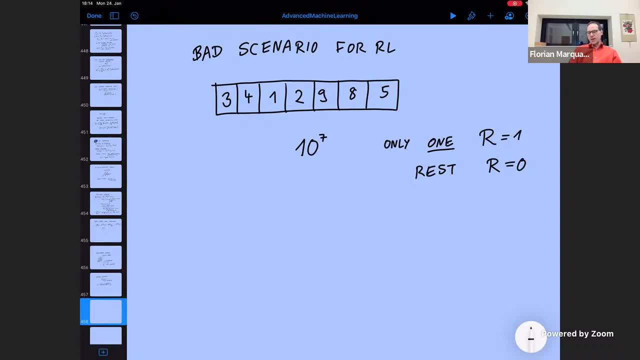 So that's the practical difficulty When reinforcement learning works. these are typically scenarios where even- let's say, to remain in this scenario- even if the first two digits are right, you already get a little bit of a reward, And if then the third digit is also right, you get even more reward. 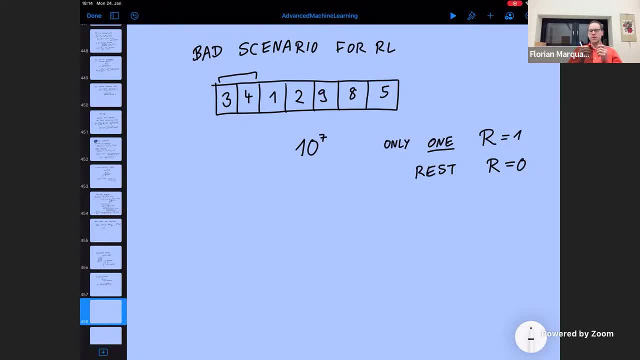 And then you can start by random guessing initially and then work your way by always following the reward. So that's the idea. So yeah, So two answers Mathematically. there are scenarios where it doesn't converge, even in principle, If you're unlucky and don't do the smart tricks that I explained in a moment. 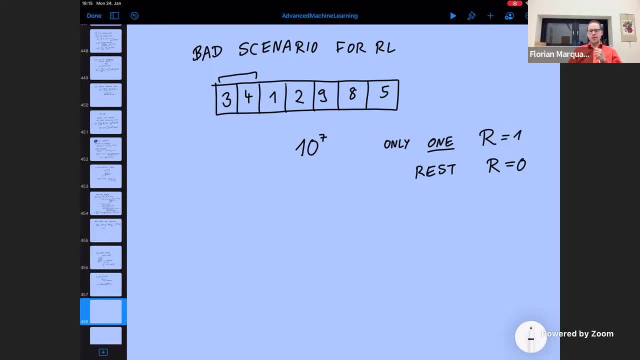 But, even more importantly, practically speaking, if you have a scenario like this where you just need to get lucky once, then it will not work. Okay, I hope. Okay, Thank you, Bye, Bye, Bye, Steve Aha. 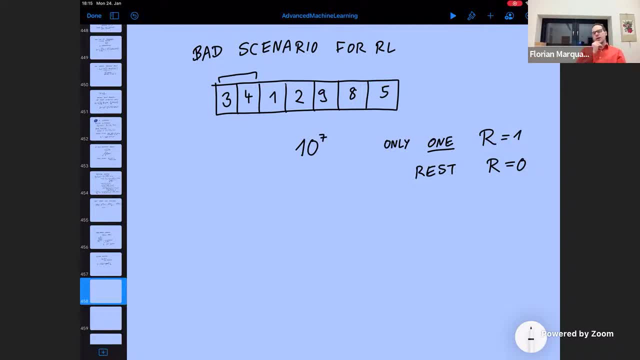 That's a good comment. This is a similar to weight initialization and neural network based gradient descent. Well, I think it's much worse than weight initialization. So in typical supervised learning scenarios, relatively regardless of what were your initial weights- unless maybe you construct a completely crazy example. 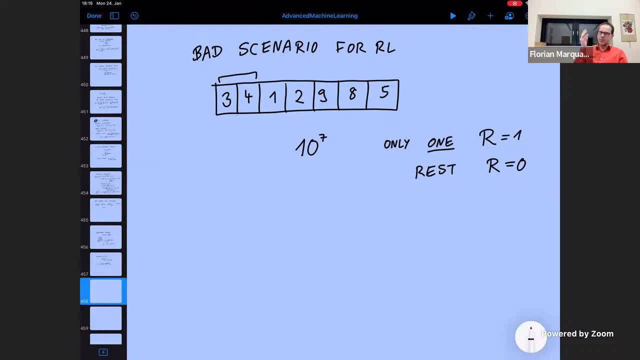 Typically, at some point you may converge. Maybe sometimes you get stuck. There's more of a between actually and very nothing stack, but then maybe you run again. so, um, the scenario i told you about here is somehow much worse, and the reason is also the if you look at the cost function in supervised learning. 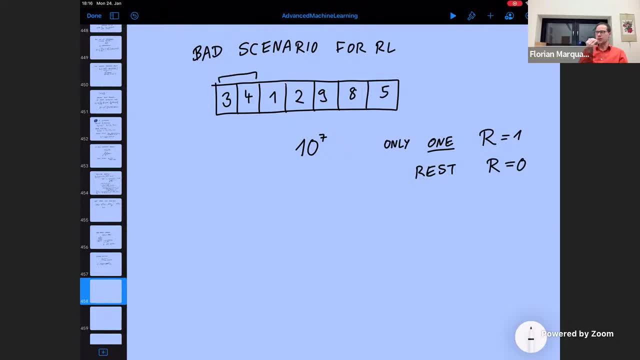 it's the mean squared error, the difference between the, the good result that you want and the output of the neural network, and even if you're very far off, what that simply means. you get a very large mean squared error, but you also get a very large gradient that pulls you in the wrong, in the right. 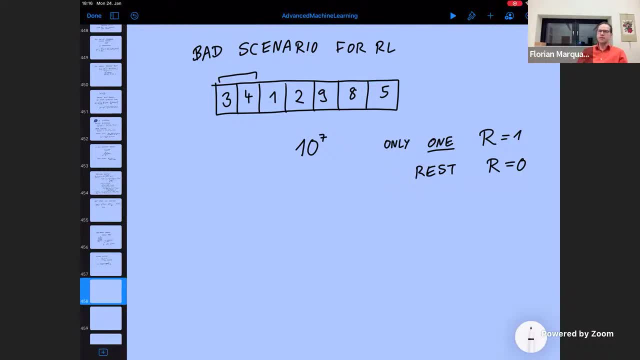 direction, and so that's already much better than what we have here, where you don't get any information if you do not hit the good sequence. okay, good. so yeah, i just mentioned already that q learning might sometimes get stuck if you're not careful and that leads to something that. 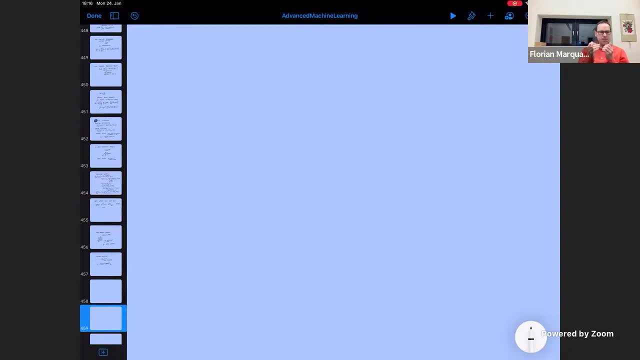 is called the difference between exploitation and exploration, so let me write it this down. so what is that? well, first of all, if the q function is very bad in the beginning, then you might get stuck, because you always try to select the action that is seemingly best. according to this: 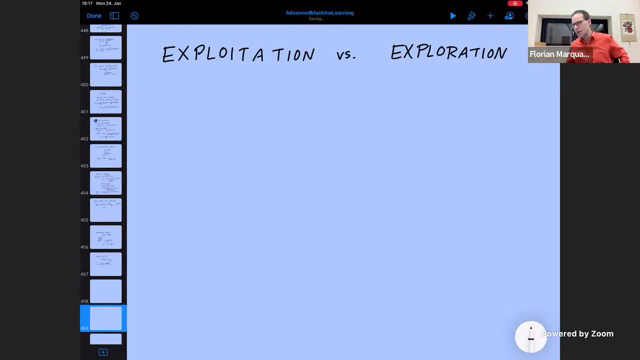 q function, but of course it's the wrong action, and then you never see what would have happened if you had chosen the good action. so that's a problem and that's why it is not good to only do exploitation, because exploitation means just to use the policy, so to select. 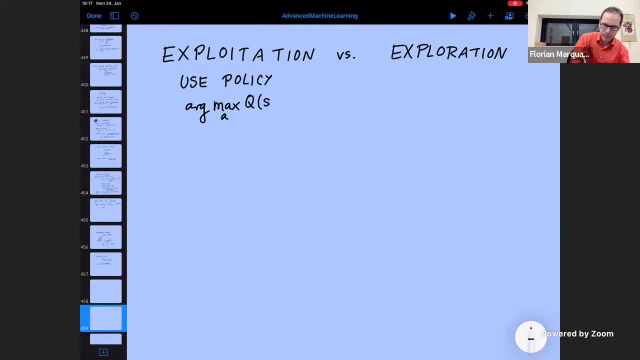 the best action, the way out of this is to do a little bit of random actions as well, so as not to get stuck always with the same action, and that's what's going on when you actually- uh, when you actually happens in exploration. so you try out something new, and the way this is often done is you draw. 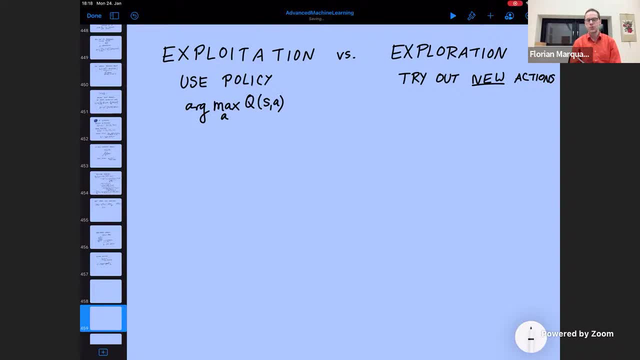 a random number and between zero and one. and if this random number is smaller than some epsilon- which will happen with probability epsilon- then you take a random action. otherwise, you take the action that is determined by the policy. and this scheme has a name: that's called epsilon greedy. 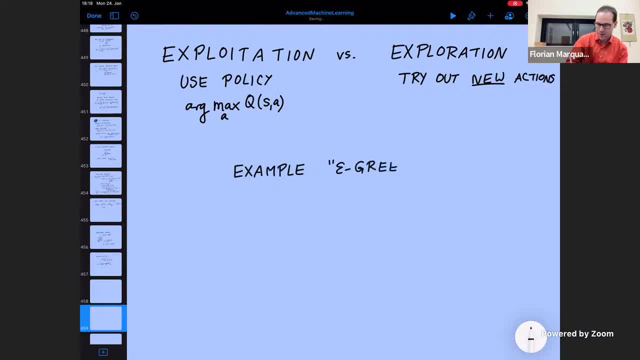 we will probably mention it a few times in the following, and it means just what i said. so with probability epsilon, you take a random action, you follow the policy and that works nicely, because at least you see a little bit of what would happen if you did something else. 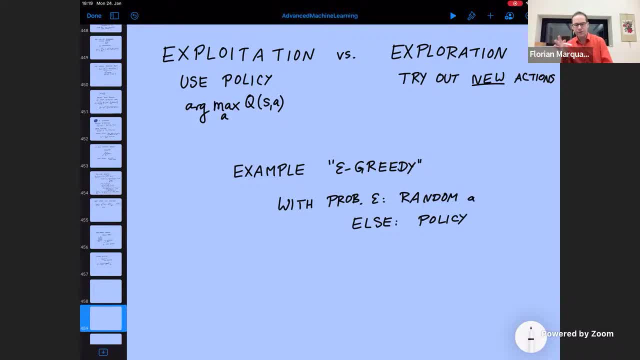 you can have variations on this theme. for example, if your q values are interpreted something like energies, you could also raise them into the exponent and you could say: my probability to take a certain action, a, i could say, is e to the q function. so that still means the higher q. 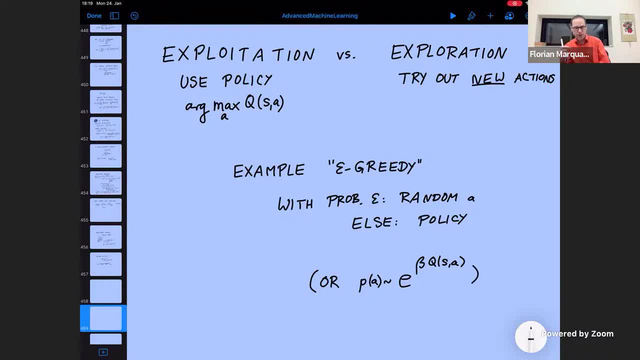 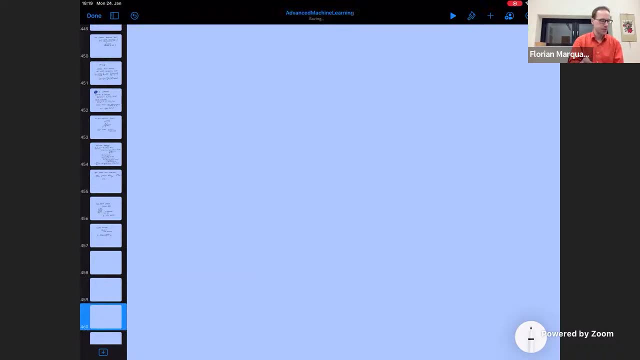 functions get preferred, but the other actions still have a chance as well. okay, so that's one thing. another topic for q learning, which is very nice because it sets us apart from policy gradient. we can reuse samples, so let me tell you how this works. so what this means is i could, while i'm going through my many trajectories, 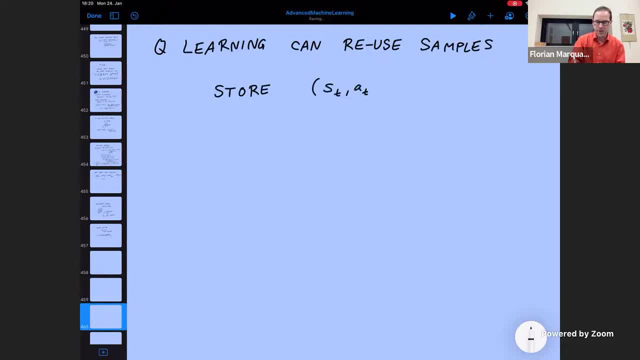 i could store the state, the action that i talk. also the state was that was reached subsequently. if that is random and the reward that was obtained, and now i can use that even later when i've already gone through many other trajectories, i can still use that to update my q function. 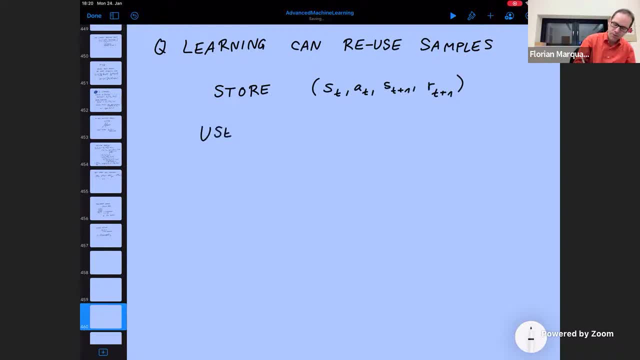 of course, i already used this particular step before, but i can use it again later on. and since i'm using an old step which is called an experience, an experience that i have made before, the whole scheme is called experience me play, and this scheme is from the working component. 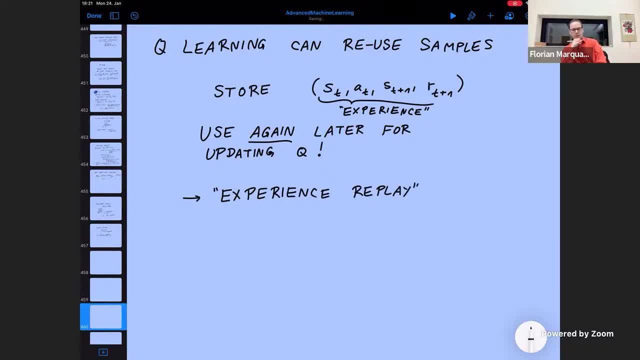 machine before. This works simply because the update equation, the Spellman equation that we use to update the Q function, that's valid for any valid state action pair, if you also know the reward. So it can always be used, even on states and actions that had been obtained previously. 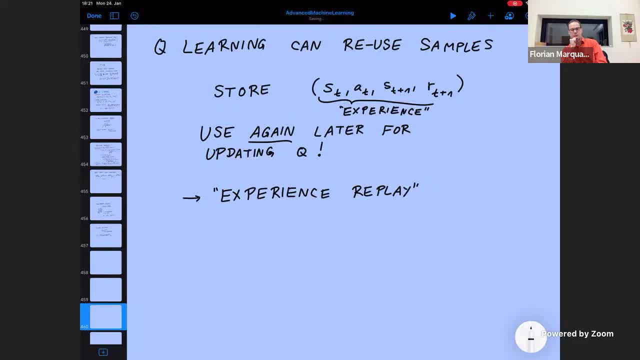 The same thing would not be true for policy gradient. Policy gradient cannot reuse old experiences, or at least not straightforwardly, And the reason is that the whole policy gradient formula rests under the assumption that the states and the actions that are written down in the current trajectory, when you take this. 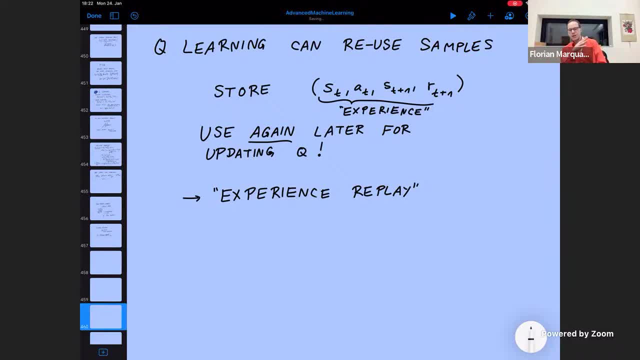 gradient of the log, of the probability and so on, that these states and actions, the sequence, was generated under the present policy. If that is not true. If these states and actions are generated under the present policy. if that is not true. if these states and actions are generated under the present policy. if that is not true. 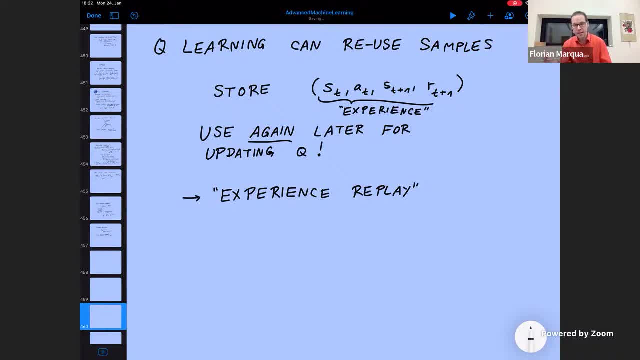 if these are old states and actions which would no longer be selected, maybe, or at least not, according to the same probabilities, then this formula is actually wrong. It doesn't work, So it's good. Here's another word that people use. 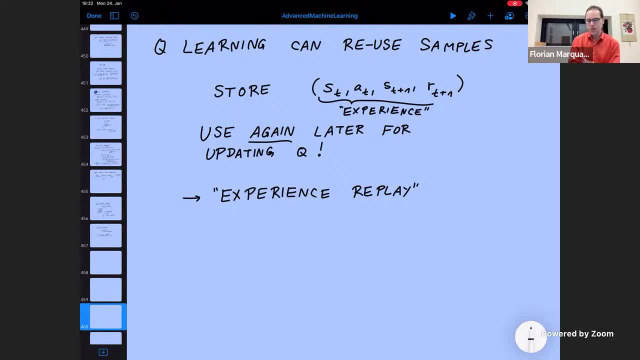 These old states and actions. they were obtained for an old policy, So by now they are, so to speak, off policy. They are not generated, maybe, by the current policy, and yet they can be used in the Bellman equation. There is no contradiction. 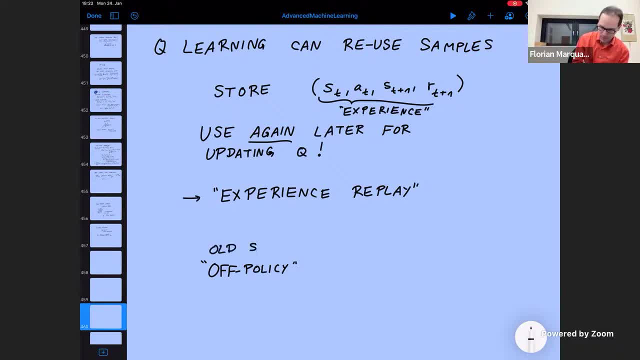 So that's the contrast to policy gradient. Let's see, So, So, So, So. that's the contrast to policy gradient. So, So, So. of course, this doesn't help you forever, because it may be that eventually you will go. 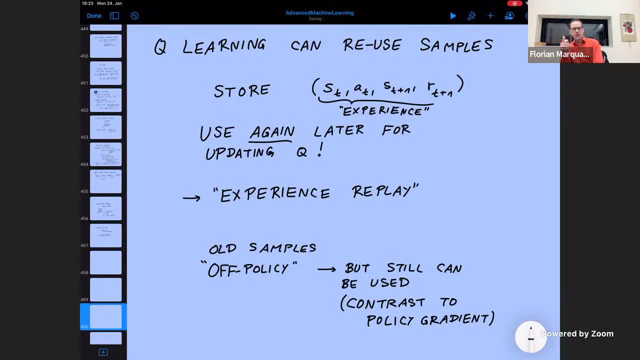 through very different trajectories, and so the states and actions that you have stored from the past, they- even though it's not mathematically wrong, still they help update the q function only in regions of state space that you will never visit anymore, and so they are not very 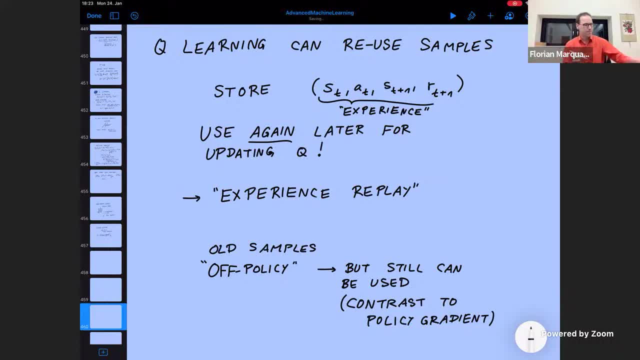 relevant in improving the current policy so that can happen. okay, good, so these were two little remarks on q learning and with that i want to finish q learning and i want to combine policy gradient and q learning and that is what is called advantage actor critic. so i told you before that. 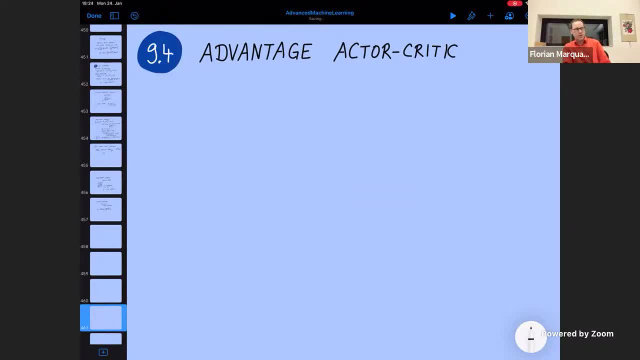 actor critic means to combine policy gradient and value-based approaches, like q learning, and the advantage. advantage refers to a particular quantity that we will introduce, which makes this even more efficient, and so these will then be the state-of-the-art approaches that people use nowadays. so let me let me start by looking at the 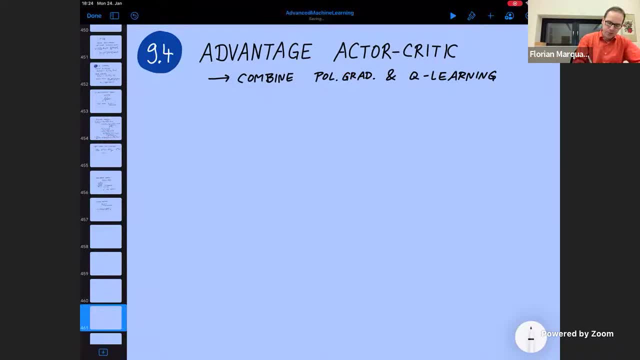 kind of expression that we use in policy gradient to optimize things. so we have contributions from each time step and at time step t. what we need is this product of the return, the future return counted from this time step, and the logarithmic gradient of the policy for that time step. 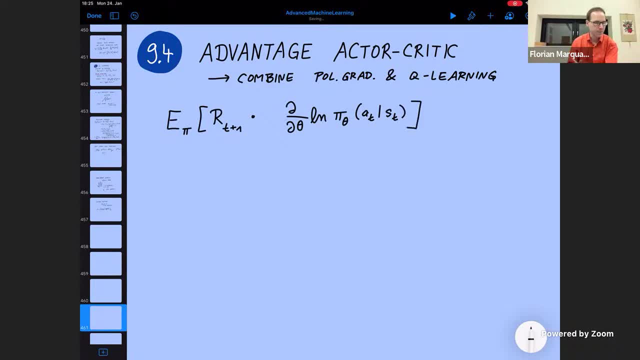 okay, and later you sum over all t and then that's your update for theta. now, what is this return? remember, this future return is the immediate reward that you get in the next time step, plus then the reward after that when you continue the trajectory and if we have some discounting you. 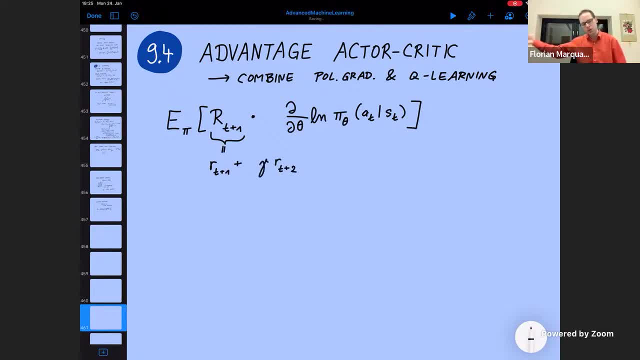 multiply this with a number less than one, because you are not so interested in rewards that are later, and then you go on. so that's the action, a function, and that is just the q function. that's the definition of the q function. now, of course, we know that the expectation value of this return itself 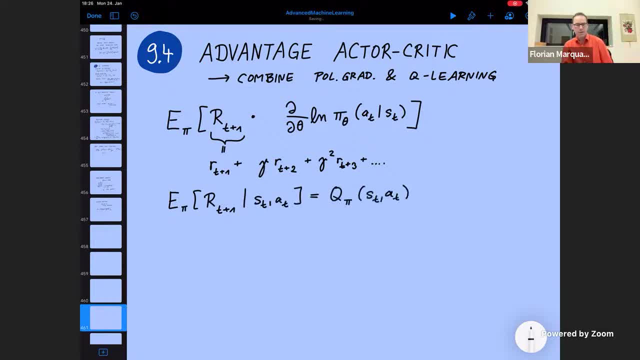 given that we are in state s and take some action. a, that is just the q function. that is the definition of the q function. question is now: can we make use of this? can we somehow, in the formula given above that we use for policy gradient, smuggle in the q function? now we have to be a little bit careful here. 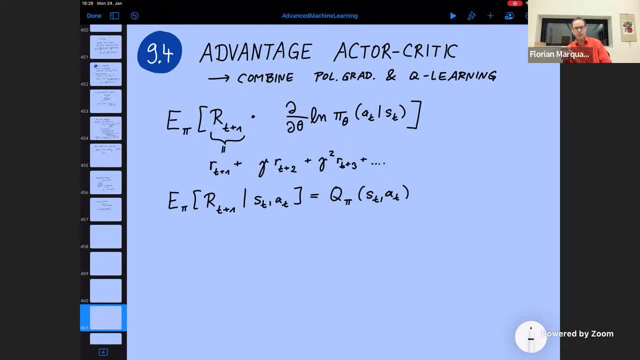 because, generally speaking, if you take the expectation value of a product, of two random variables, like here, return times, this logarithmic gradient, so if you take the expectation value of such a product, you cannot simply, without thinking, replace one of the factors by its expectation value. that would be wrong in general. but here the situation is a little bit special and i 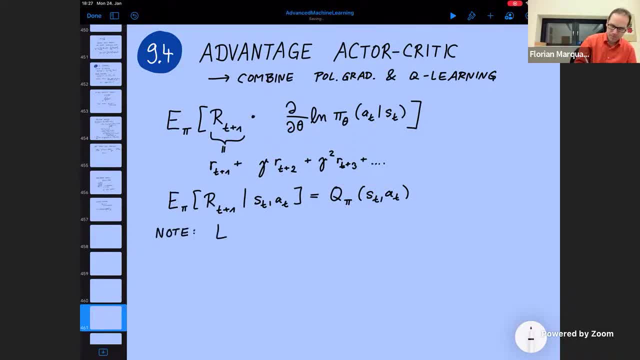 maybe write it down best in a more generic way, then you see what is happening. so imagine, i have two random variables, let's call them x and y, and i have this product of functions of x and y, so f of x, comma, y times g of x. so now there is a trick i can do. 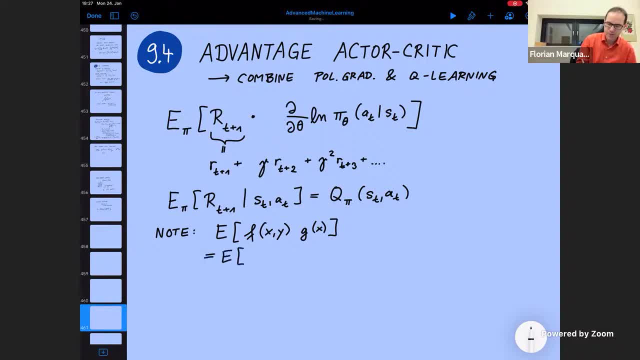 i can say this is the same as the following expectation value: i first consider this f of x comma y, and i hold x fixed, and then i take the expectation value of this quantity, that is, i average over y, obviously given a fixed x, and then i multiply the result with: 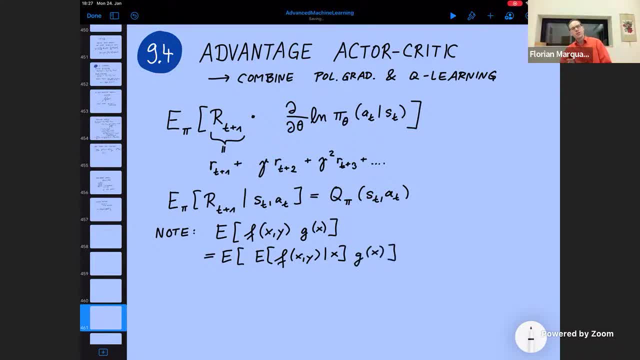 g of x, and then i take the expectation value of this quantity, that is, i average over y, obviously, and then i multiply the result with g of x, and then i take the expectation value of this quantity of x, and then i average also over x. so this is a correct statement, and so now we can apply the 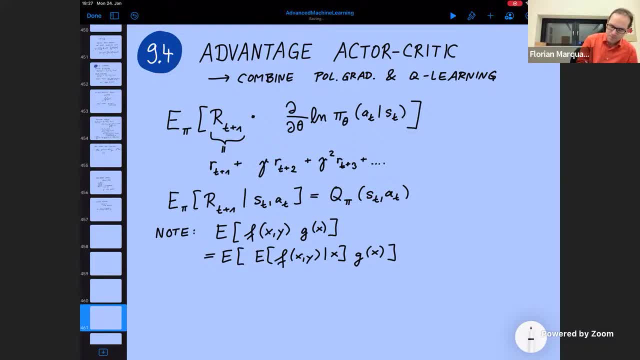 same to our situation because, you see, what i have here is something that only depends on the current state and action and nothing else, and another factor- the return- that depends also on the state and action and what happens in all the subsequent steps. so it's a little bit like this: 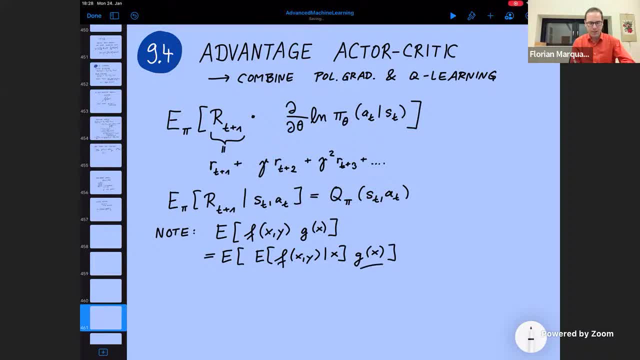 g of x would correspond to the logarithmic gradient, and the f of x comma y corresponds to the return, and so i can play the same trick. so let me continue here. the expectation value that we need for the policy gradient is then indeed just the same as if i would. 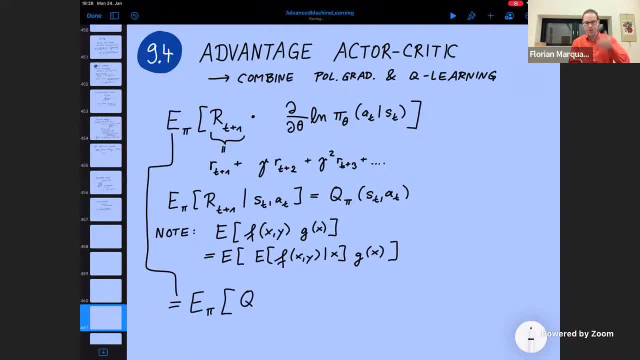 take the conditional expectation value of the return inside the brackets, and this conditional expectation value is just the q function. okay, and so that's the whole trick of how to smuggle in the q function into our policy gradient. and now you can imagine that this gives opportunities. namely, you can use any of these bellman type update equations to get very good. 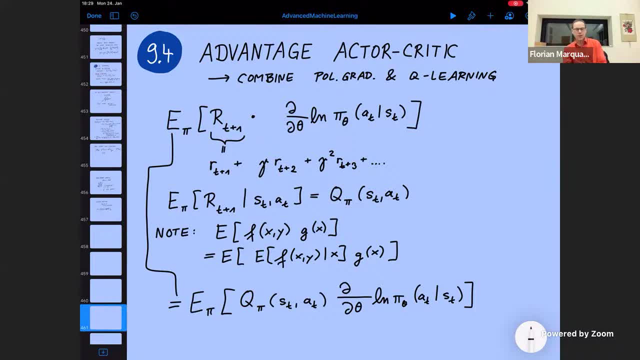 estimates for the q function and then you can use them here, and it may make your estimates for this policy gradient much more stable, because the q function is already an average value that has been updated using the self-consistency equation. it has little fluctuations, whereas if you had 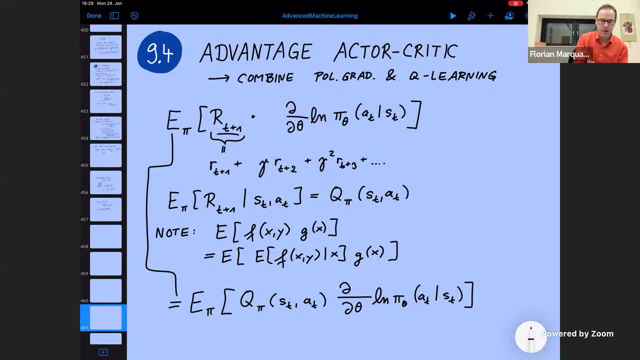 just naively taken the monte carlo evaluation of the return, so just running the full trajectory and noting the return even for a small batch of trajectories that has much bigger fluctuations. okay, so that was the first step. we smuggled our q function into the policy gradient and now we can take one step. 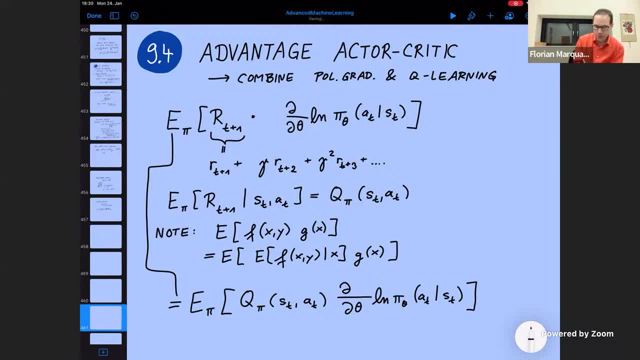 further and we can try to further reduce the variance of this whole thing and we've already learned a technique of how to do that. we said, if we take whatever is here, in the old days it was just the return, now it has become the q function. if we take that and subtract any function of the current state, 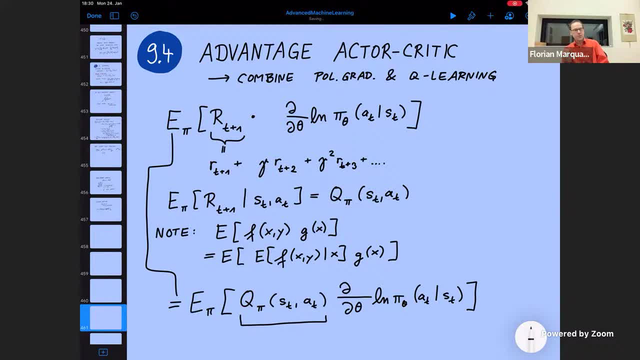 the overall expectation value remains the same. that doesn't matter, and so we call this a baseline. the question is now: which point is the most important point in the equation and which point is the most important point in the equation and which point is the most important point in the equation? 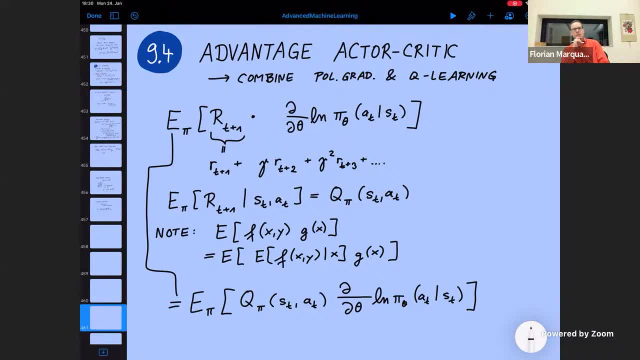 and which baseline would you choose? well, it would seem a good idea to subtract from the q function something that is equal to the average of the q function, such in such a way that it only depends on the state, because if that is the case, then you expect smaller fluctuations. so, um, how do we see this? 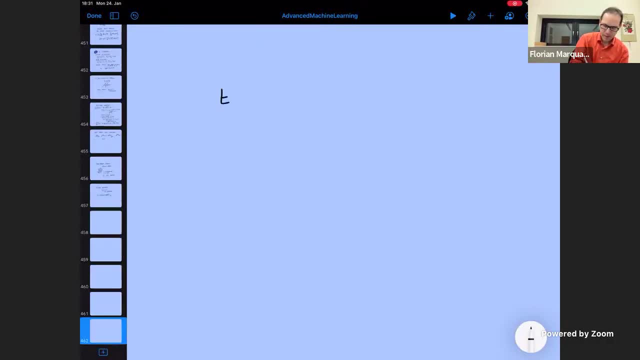 let's say so. we want something like the q function minus a suitably chosen baseline times. this logarithm, the gradient of the logarithm, has the same value in expectation as if you only had the q function. so that's already a given um. but we want to choose the b. 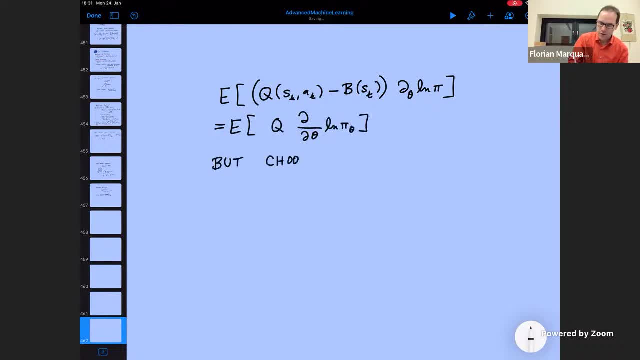 to reduce the variance of the whole estimate, because after all you will not do this expectation value really by going over all infinitely many trajectories, but you only have a handful and then average over them. so you do it by sampling and then it would be bad if the fluctuations 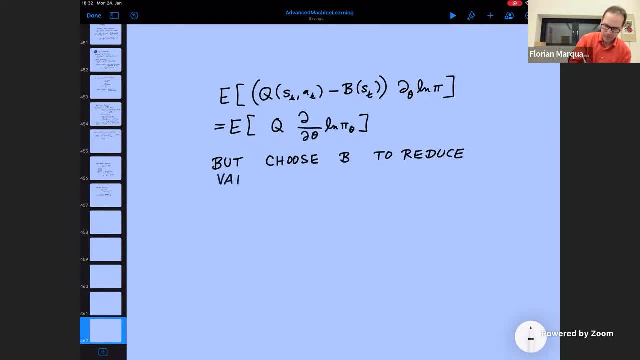 uh, are too big, And so the idea here is to choose the expectation value of the Q function given a certain given the current state s. But what is that? Well, by definition, we have done this before, or you can look up the definition we had before. this is: 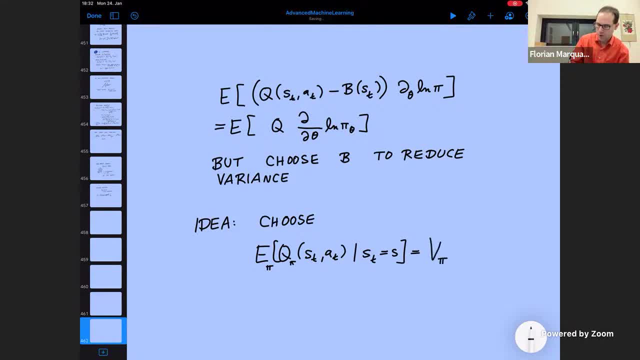 just the value function. So if you say, let me average over all possible actions I could take, This is just the value function. Okay, good, So let's do that. Let's subtract from the Q function its average, namely the value function, And then we 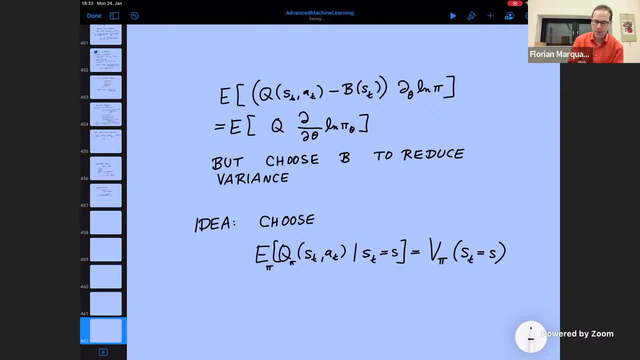 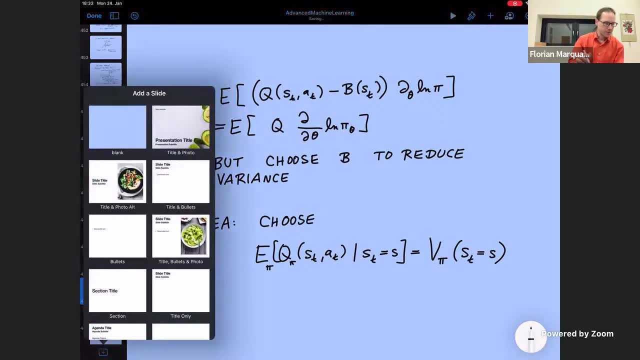 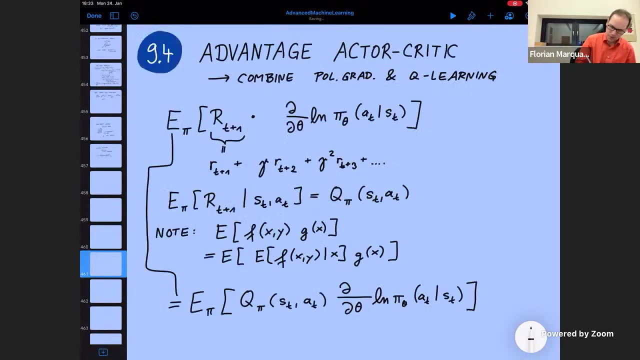 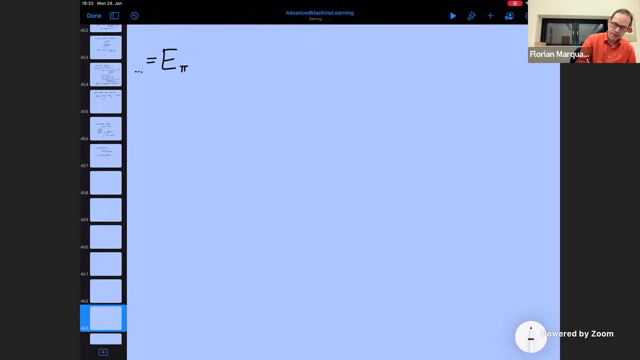 over all can expect to get a reduced variance for this whole estimate of what we need for the policy gradient. And so that that now leads us to let me see, So I will continue here. We say, whatever we wrote up there is the same as this difference. 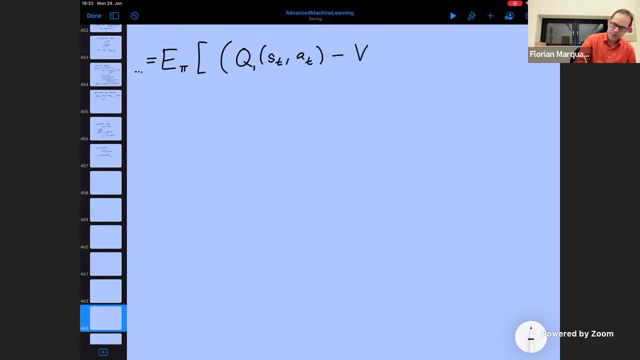 between the Q function and the value function, And this thing has the name That is called the advantage. So we will call it a of s T 80.. So what does it mean? what does this advantage mean? It means, if you select this particular 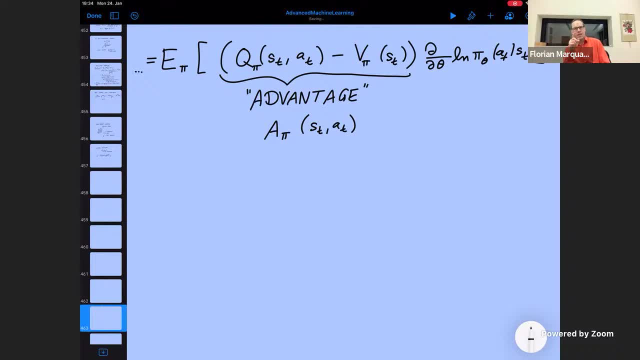 action A: are you doing better than what you expect on average, given the current policy? If yes, then of course that's a sign that you should prefer this action of over whatever is taken in the current policy. And if no, if the advantage is negative. 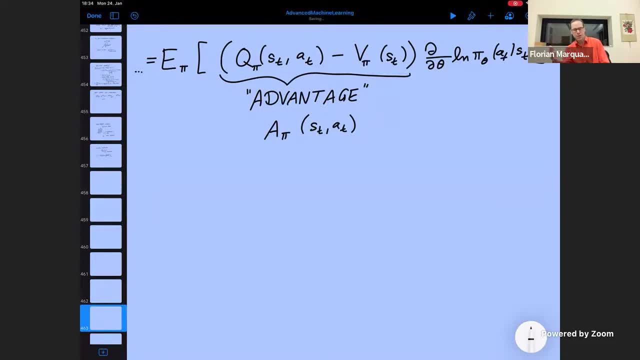 then that means this particular action, AT, is actually worse than what the current policy does on average. So how much better does this action perform than what you would expect on average from the current policy? Okay, So it's very obvious that this is a very good quantity to look at. 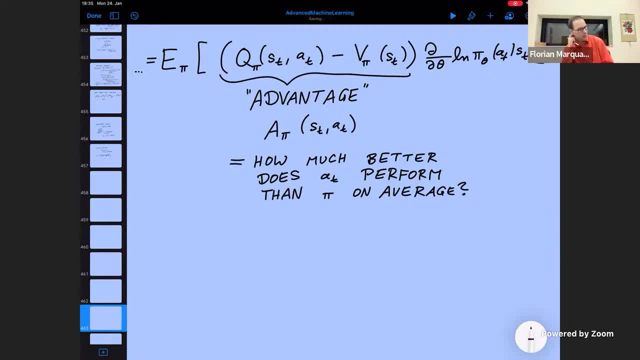 And here we see how it came in automatically in our policy. We see gradient update. Now there are interesting observations to make. The first thing: what's the expectation value of this advantage? So you keep the state fixed and you look at the advantage. 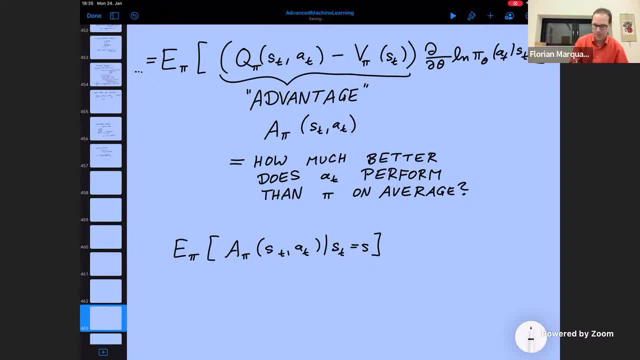 You take the expectation value over the policy, And if you insert this, then of course you get the first term. the average of Q will just be V again, And the second term was already V. so what you get is zero. So on average you don't have an advantage. 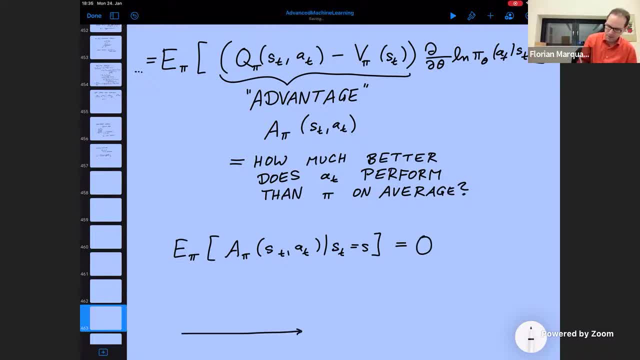 And so the way this looks like is like here. So let me plot the advantage on the x-axis And then on the y-axis I will put the probabilities of different actions that we could take. Let's say there's a disadvantage. 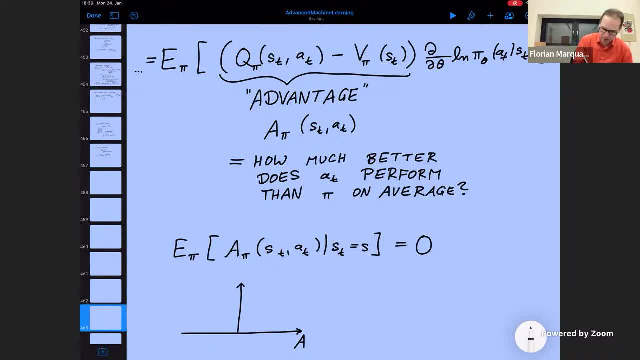 There's a discrete amount of actions. Let's say, there is one action here which occurs with a certain probability and which has a negative advantage- Okay, so it's a bad action- And then there is another one which has a positive advantage, and maybe yet another one which also has a positive advantage. 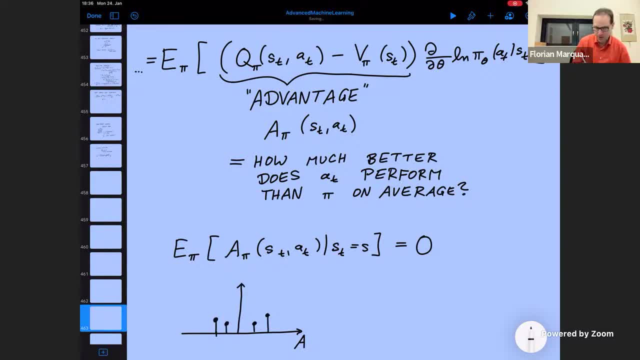 and yet another one which also has a negative advantage. So what this formula means is that if I take the, the average over all these different actions, then yeah, then I get zero. So the weight of the center of this distribution. 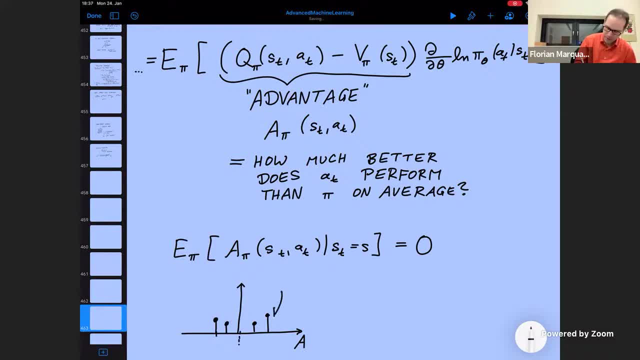 must lie here. So what I was plotting here were the probabilities of these particular actions given the current state, and the horizontal was just the advantage that I get Now. this is obviously a policy which is not yet optimal, because there are actions that have a positive advantage. 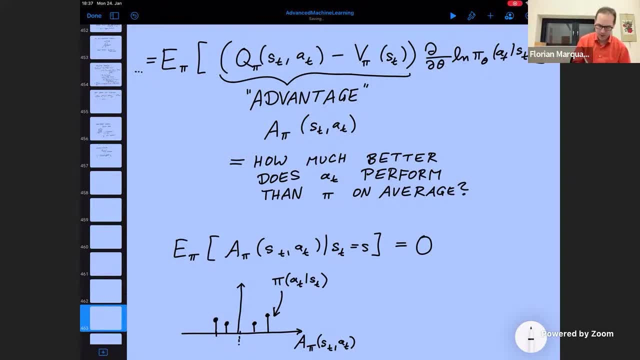 which means they are better than whatever the current policy tells us. So this is when the policy is suboptimal. So how does it look like if the policy is actually optimal? Well, in that case I still must get zero on average. 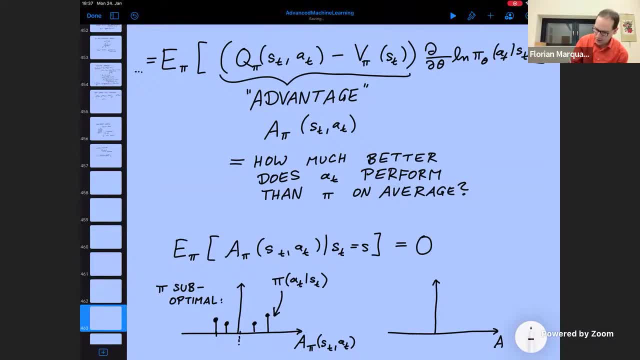 And the only way this works is that only one action is selected, or at least there's only. there's only actions with this zero advantage. There's sorry, there's of course also other actions. they lie here, but they all come with zero probability. 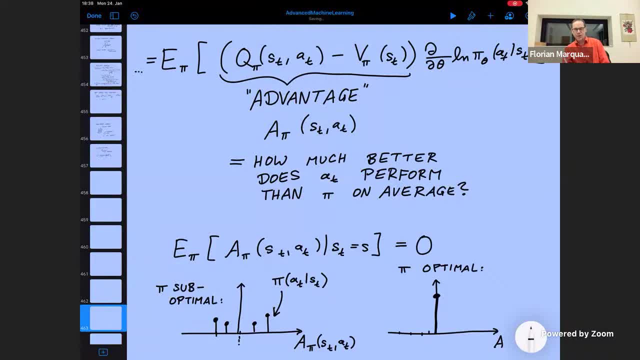 If they did not come with zero probability, then this action that I now draw right here in the center would have to shift a little bit to the right in order to make the average advantage zero, And that would mean there is one action then that has a positive advantage. 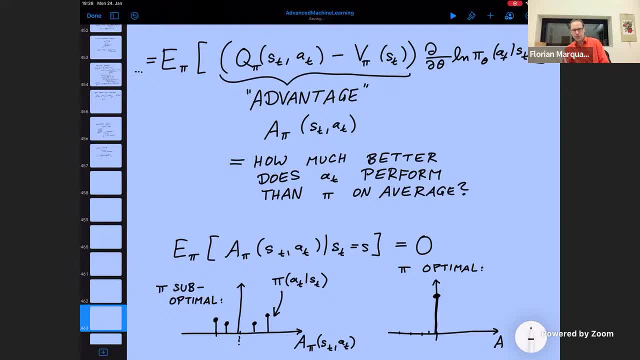 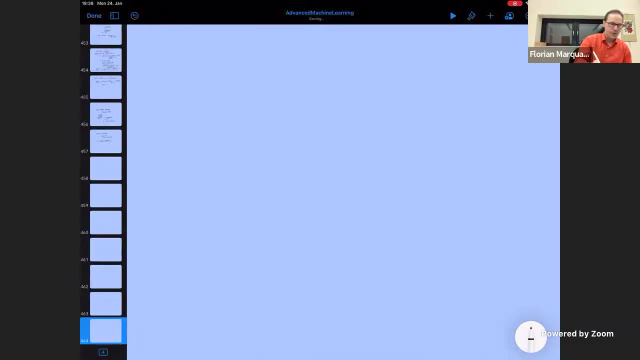 which would mean that the policy is not yet optimal. So if the policy is optimal, the picture is simply like this and there's only zero advantage. Okay, so let's summarize things. We will now use policy gradient in this advantage. actor critic style. 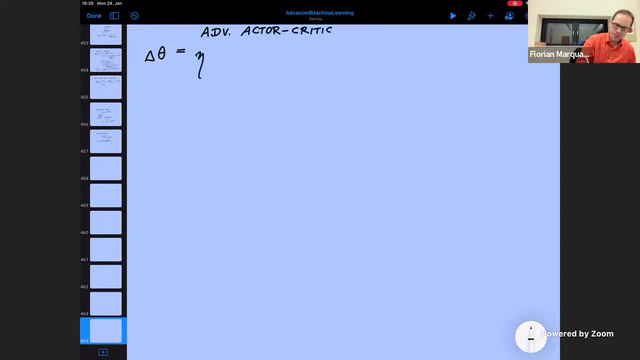 That means the update is some learning rate. the sum over all times times the expectation value of this advantage, times the logarithmic gradient. Okay, fine, So now how do we approximate the advantage? I already told you even when we started. 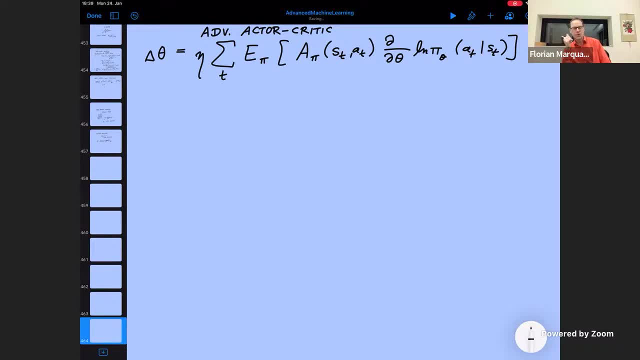 we would use something like a Bellman equation to find the Q function or whatever we need. By now we have turned it into the advantage. The question is, what's a good approximation for the advantage? So let's take an estimate from some trajectory. 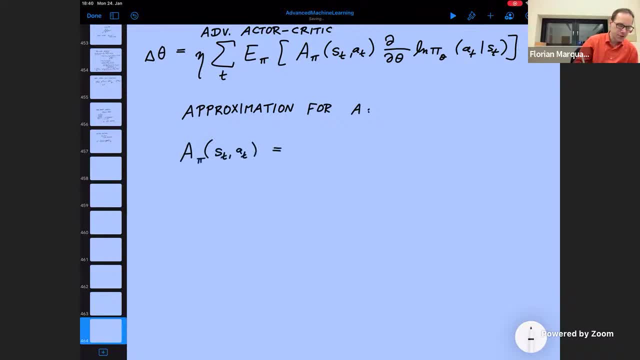 Let's take an estimate for the advantage And we could say, well, we follow this, then Bellman equation spirit, And we just say, well, the advantage is, let's say the, a good estimate for the Q function minus the value function, which we also have to estimate. 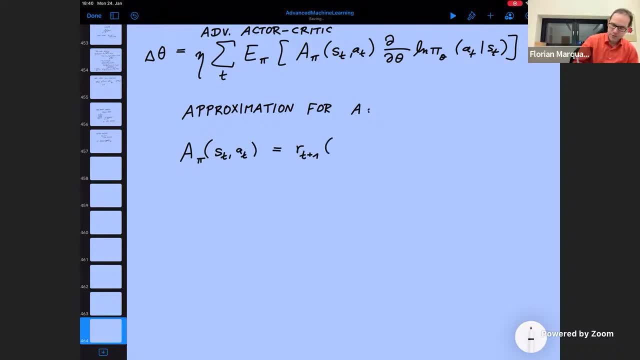 And so that would be a good estimate for the Q function is if we take the reward for the next time step where we add gamma plus the measure plus gamma times, the reward for the next time step depends on blah, blah, blah, blah. 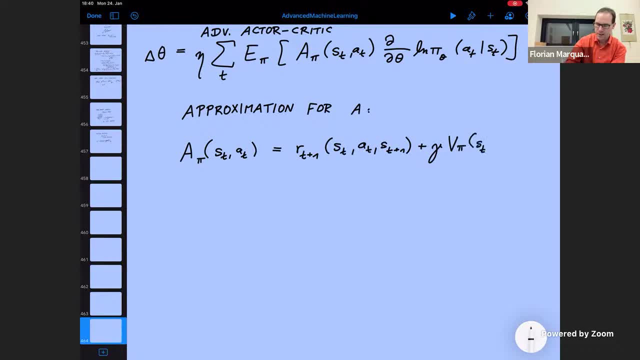 But that can then be replaced by the value function starting from the next time step. We're not interested anymore in the details of how the sequence is carried out further, And that would just be a good estimate for the Q function. We subtract the value function. 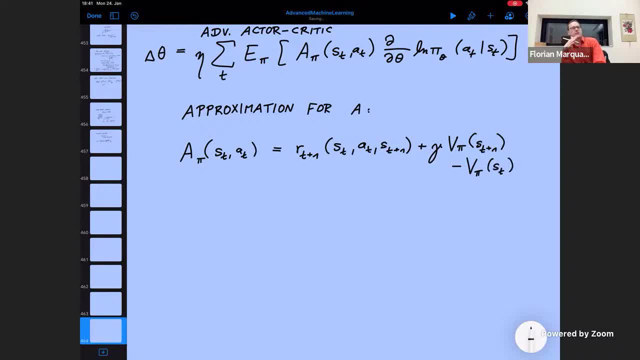 at the current state, because that's the definition of the advantage. see again, this is a quantity that will not fluctuate too much. Sure, there is the reward. that depends very sensitively on the current action, But then wherever we end up with in, 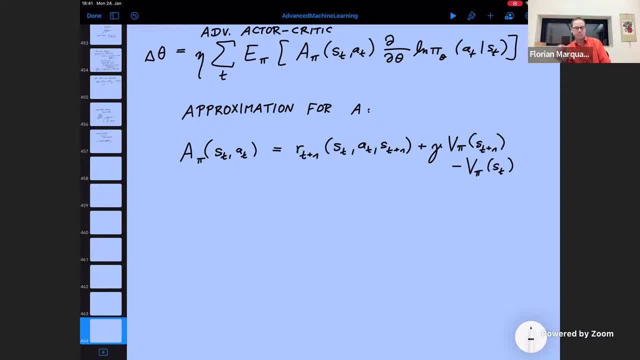 which state st plus one. we end up, we just exploit that we maybe have a good approximation to the value function. Okay, so just quick remark, side remark, you could also continue this. So instead of just writing the reward, rt plus one, you could also write plus gamma, rt plus. 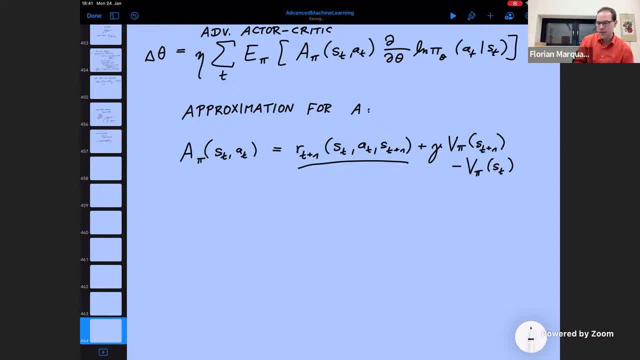 two plus gamma, squared rt plus three plus gamma to the third times the value function at this st plus four. I suppose that you have then. So there are different versions of this approximation depending on whether you trust your estimate for the value function already or not so much. 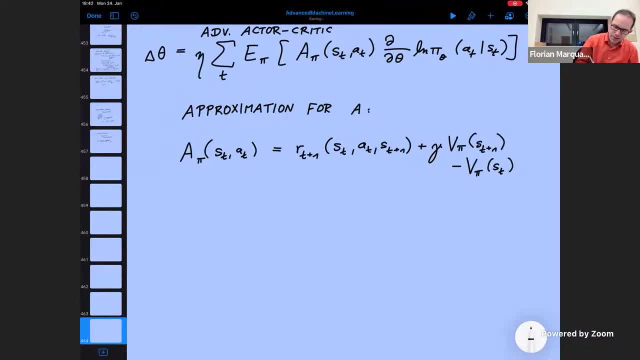 Okay, so that was it. So that was one remark. Then how do we get the value function? we still need the value function, And what we just use is the Bellman update. So we would say that the version of the Bellman update for the value function. we only wrote it down for the cube function. 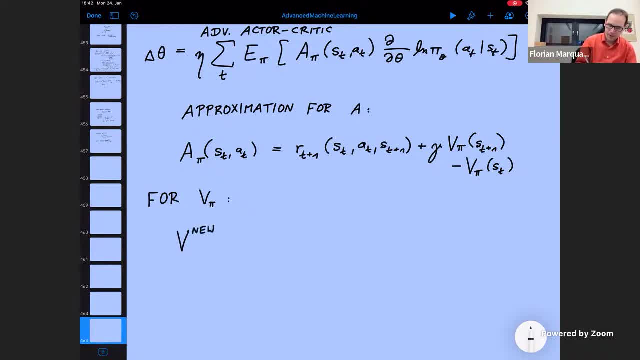 so far. So we would say, as before, the new value of the value function is the old value plus the update. And the update, if you write it down, for this case, would be this: immediate report times, gamma times, the value at st plus one minus the value at st, And now you'll see something funny. whatever is written, 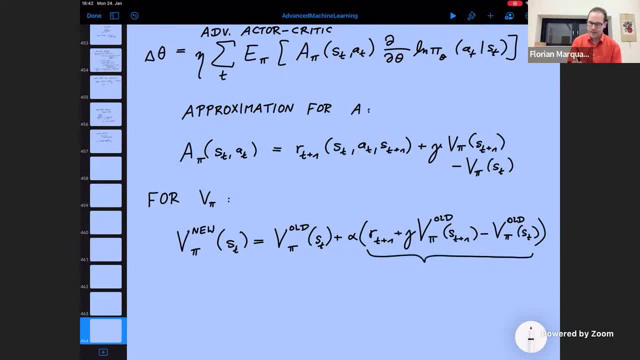 down in this bracket is exactly the same thing, the same expression, that we already had a factbrate. Let's simplify this by saying: this string equals a library here. Okay, Gone, This is really a weird things laying in there for me, Okay. 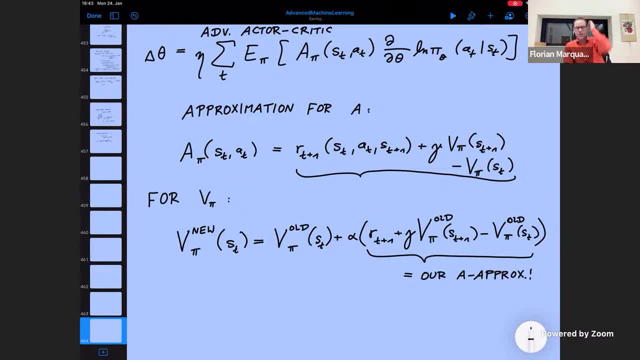 Let's try one more. Let me just close that one. And so this is how advantage actor critic works. You are updating at the same time your value function and from that you always get the advantage for any given action, and it is that which you use to get your policy gradient. 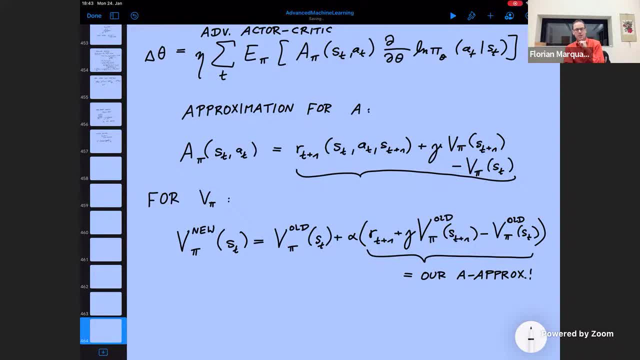 updates. Now how does that work in practice? You could have a small state space, in which case the value function could be written down as a table, and you would literally do this update for every state at the same time. You do a table based approach, maybe. 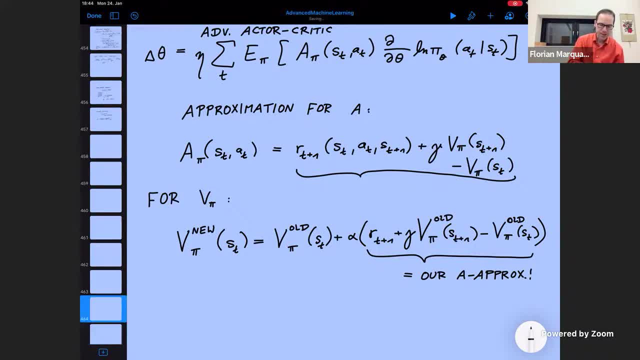 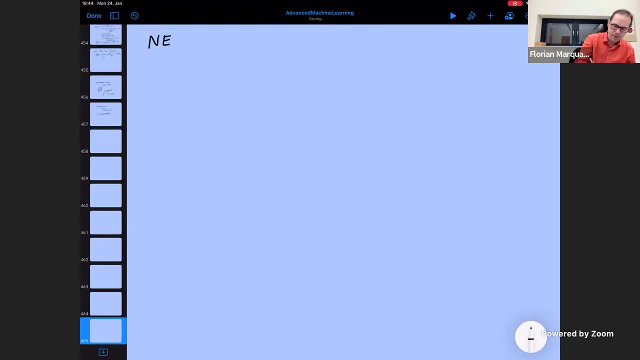 You could do that, but if the state space is larger, you have to have something more advanced. You need a neural network, Okay, And so what you would do is what I explained before. for the Q function, for example, you 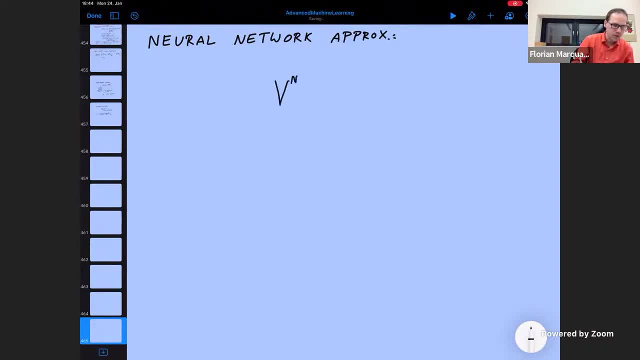 would say: let me calculate the value of a given state using a neural network. Maybe let's call the parameters mu, and I try to match as closely as possible whatever I got from the table. Okay, So let's do a fixed point equation from the Bellman update. 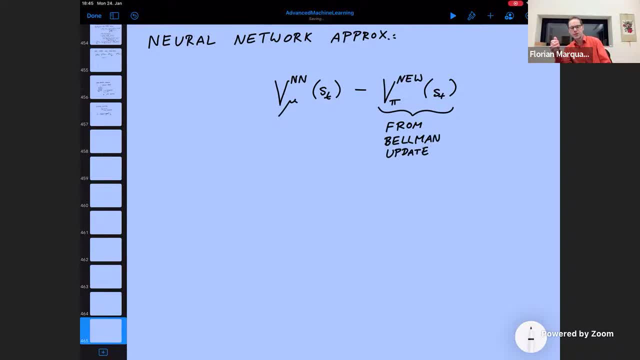 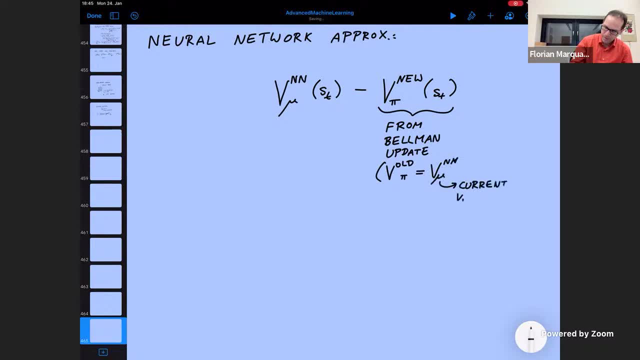 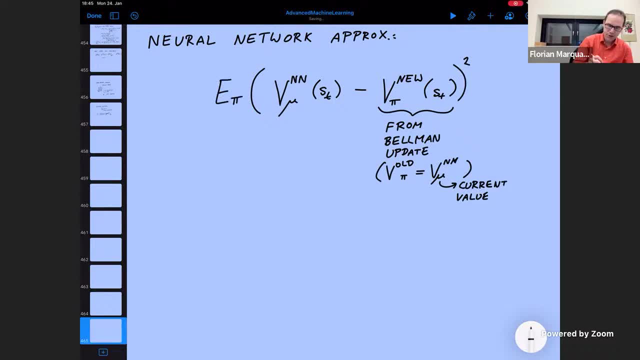 And probably you should sum over all times in the trajectory, And so this is how it's all coming together here. Okay, So you can I spend more testing time, which is a great debate. really is how you would get your value function. 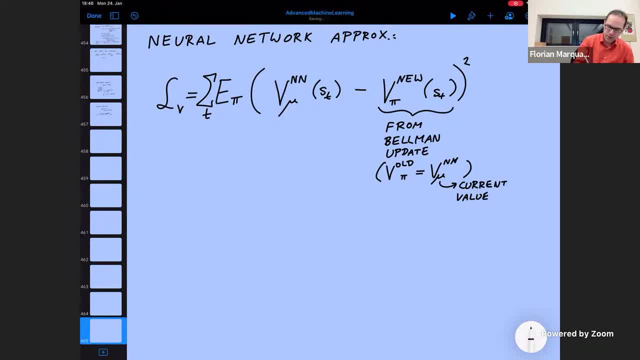 Now, in that spirit, then there are two networks, apparently. There's a policy network which tells you, given the state, which action should I take, And then there will be a value network which tells you, given a state, how good is that state? 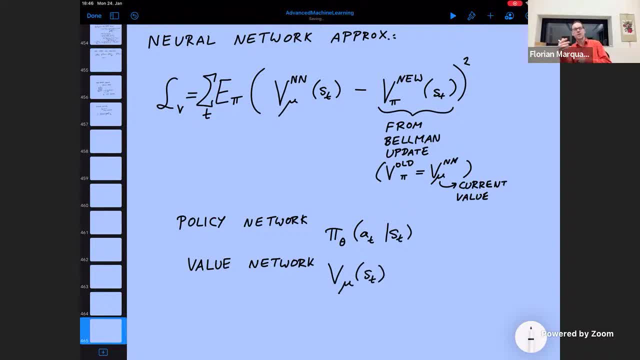 And so you're learning both at the same time. You're improving the policy with policy gradient, but you're also improving the estimates of the value network, And that is used for the advantage that enters the policy update. Now, sometimes, of course, you realize the state. 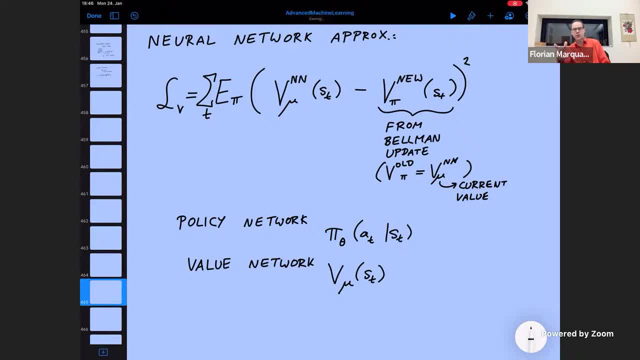 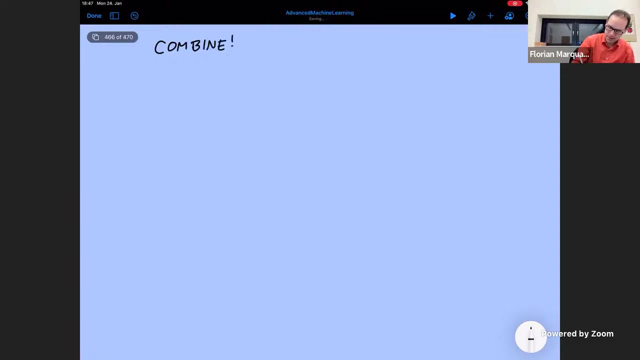 that you send in here may be as complex as an image, a whole high dimensional image, And so people found it smart if, instead of just having two different networks, you would reuse the same network, and the way this can work is the following: So you would say: I have my state. 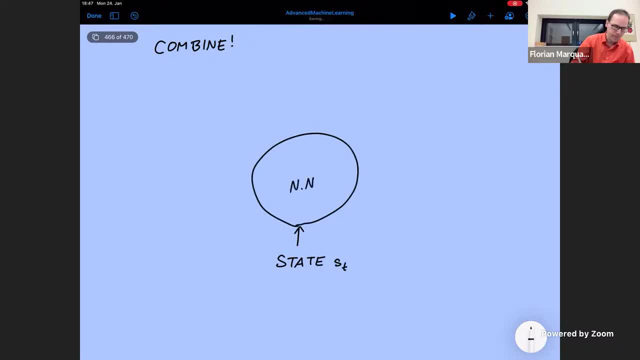 I send it into my neural network And then this already does all the complicated processing of the images, maybe a convolutional neural network and so on, And then it has multiple outputs, which just really means that, say, you have 10 output neurons and three output neurons. The first three I define as one part of the output. 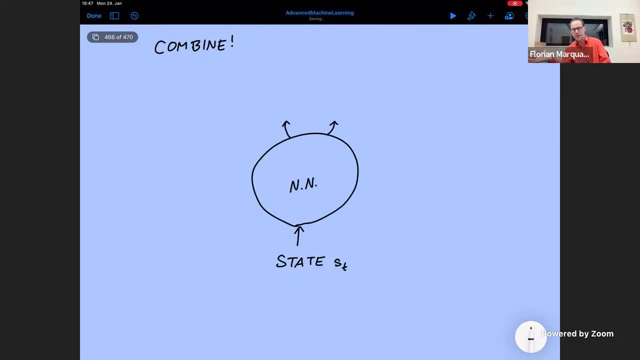 and the other seven remaining neurons I define as the other part of the output. So this is what we mean when we say it has multiple outputs, And then you could take one part of the output. Sorry, this was not quite right, So you may just take the full output. that is, so to speak. 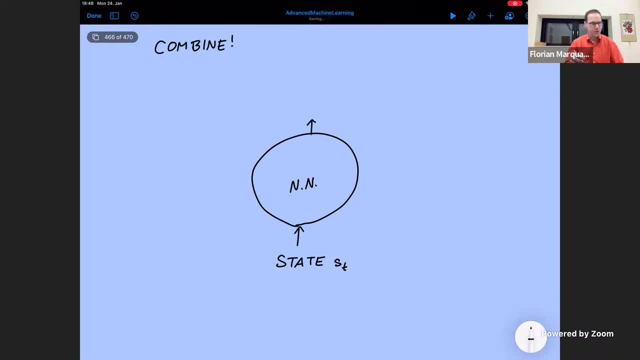 a representation of the state, which is already compressed, which has a small number of neurons, And you feed the same output into two different networks. There will be one network which eventually produces the value, So it only has a single output neuron. 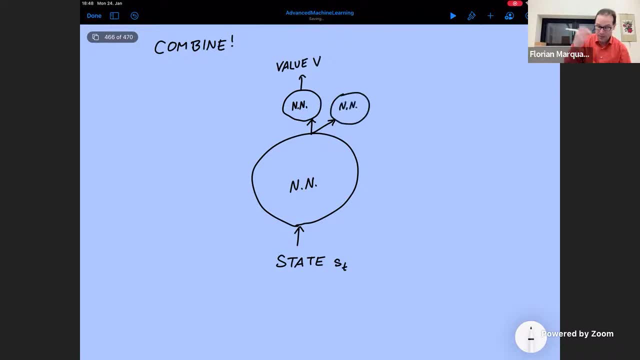 And there will be another network that starts from the same state representation but has a different task, namely to predict what is the policy. And again, the policy is typically a probability distribution over different discrete actions. So you have a finite number of output neurons corresponding to the finite number of actions, And so this now becomes the 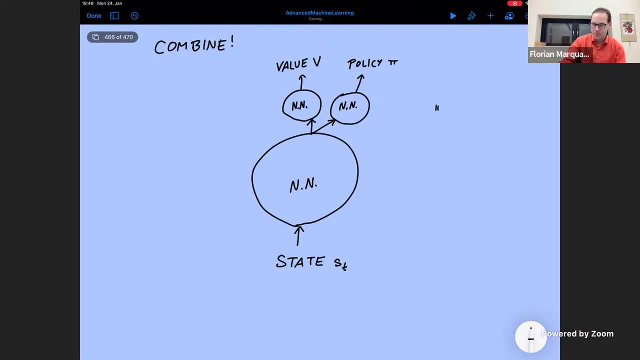 overall neural network And the language that people use is that this network has two heads. So you will have a body in the lower part that does the heavy processing of the image. let's say that represents the state, And then this is being fed into the two pieces that 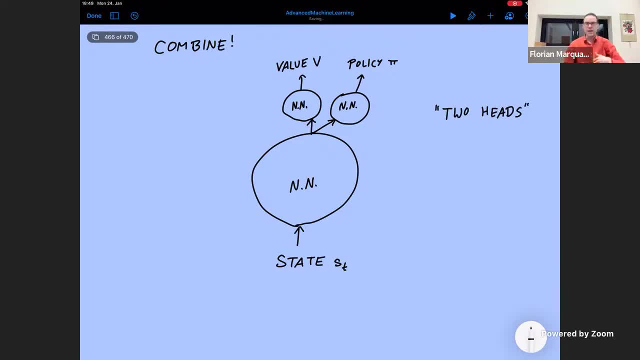 will predict the value and the policy. And now you can say that theta would represent, say, all parameters in this whole neural network, a network including all its pieces, all its head. And so then what you could do is you write down a loss function, which would be the kind 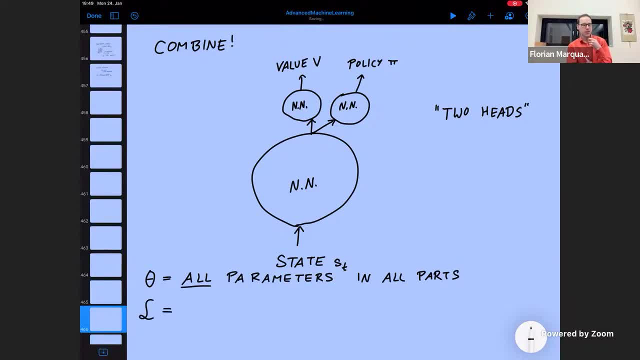 of loss function that you would need in order to get the policy gradient updates with the logarithms and another part of the loss function, that is the loss function that we used for the update of the value network. So you would write down something like maybe this sum over all time steps: advantage times. 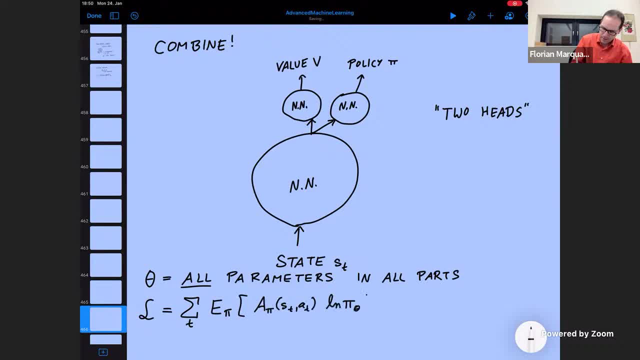 log pi theta. So this is the first part of the loss function. It is supposed to give you the proper policy gradient update. For the policy gradient update, The gradient should only act up the logarithm. Now, in principle. of course, inside this action we also have the value functions. that also. 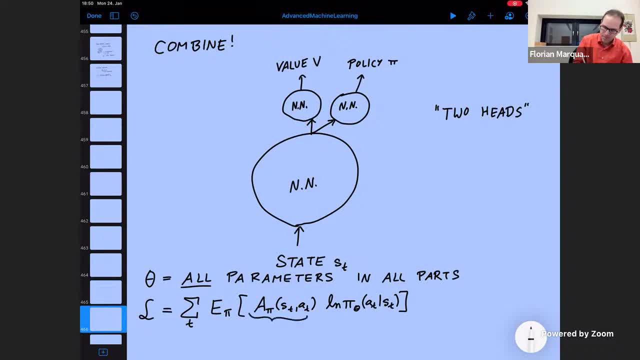 depends on theta. This part we should not differentiate, So theta should be fixed inside here. Plus, then we have the loss function for the value part, which we discussed before. Only now, And I would say, instead of mu I can just use theta. 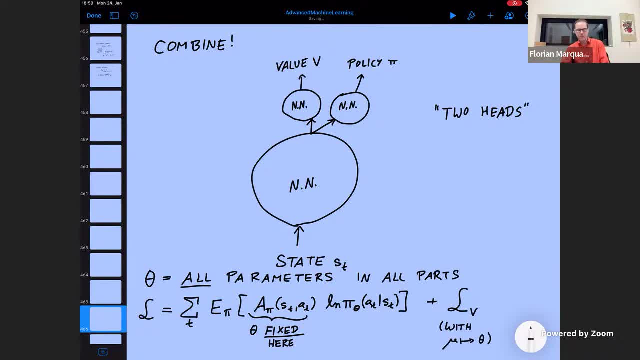 Theta describes all the parameters of this network structure, And so this is then how people really use advantage: actor critic: Okay, So any question about this. So having a value function is also very nice in order to be able to interpret things, because 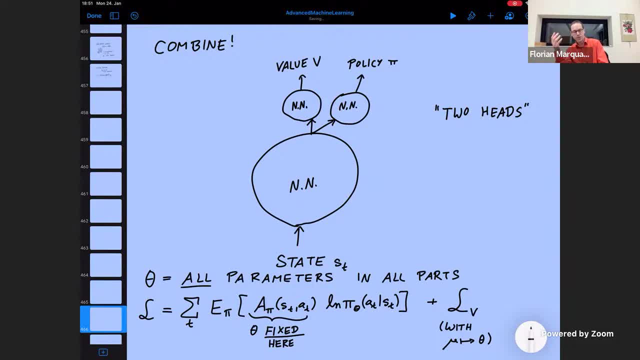 then, for different states, you can plot: what is the value, what does the network think is the value of that state. Okay, so now this, let's say, was the state of the art a few years ago, But then things evolved a little further still. within this advantage-actor-critic idea, 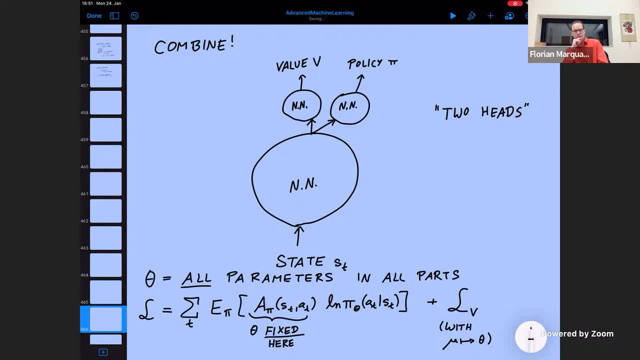 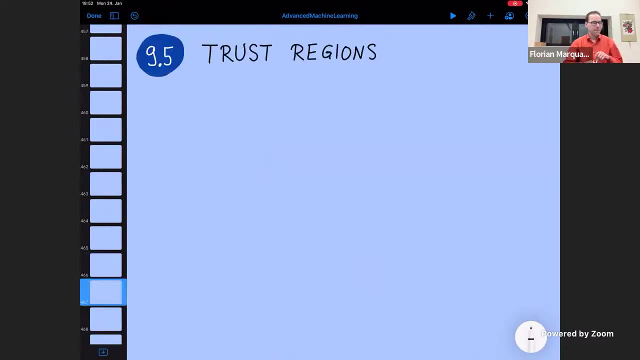 but with some smart ideas about how to take larger training steps. So to make the updates in the theta parameters. I don't want to make too small updates And that's what I'm going to discuss next. So the headline here sounds a little bit mysterious, but trust me, it will make sense in a moment. 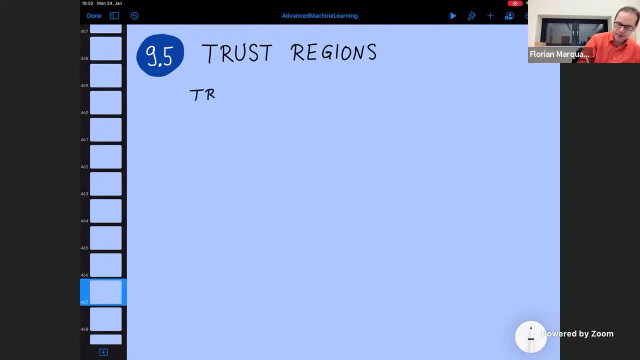 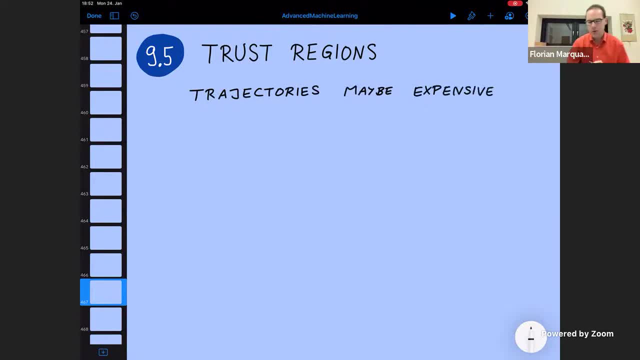 In a real world that's not the case In a real world environment may also be true if the simulations that you're running on a computer are expensive. So it is in your interest that you do not need to have too many trajectories and that for all the information you acquire, you make relatively large updates of the policy. 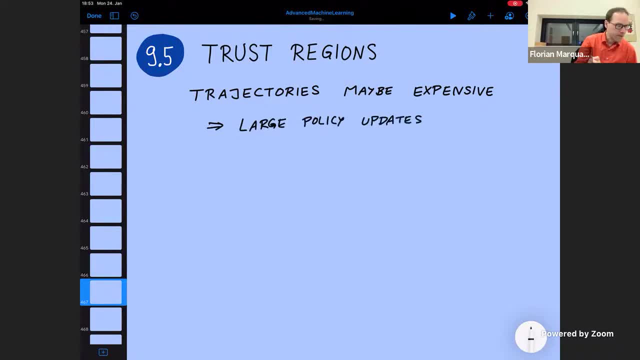 and that, for all the information you acquire, you make relatively large updates of the policy. So the picture you should have in mind is: here is parameter space. So the picture you should have in mind is: here is parameter space. Here is maybe your current parameter. 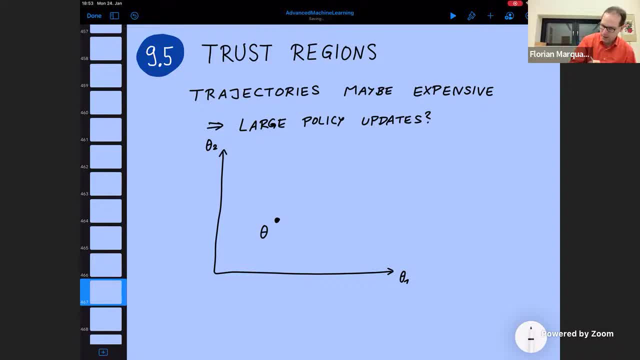 And then you can do several things. You could do just a small update following the gradient. You could do just a small update following the gradient, But then you can do a little bit more. But then you can do a little bit more And then resample again some trajectories and update again, and so on. 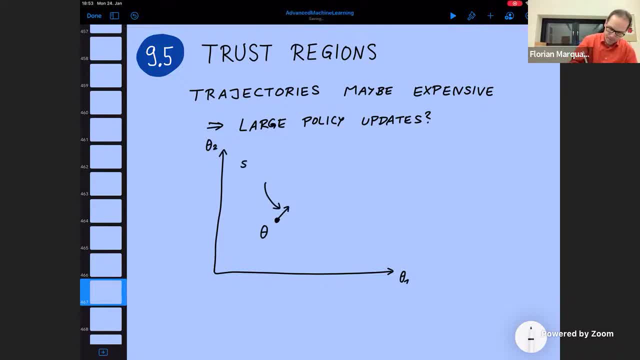 But that will be expensive. Okay, so that's expensive. You could also simply say: oh no, I take my learning rate really large And I will just go in the same direction and take a really large update, But it's almost certain that this is not the correct direction anymore. 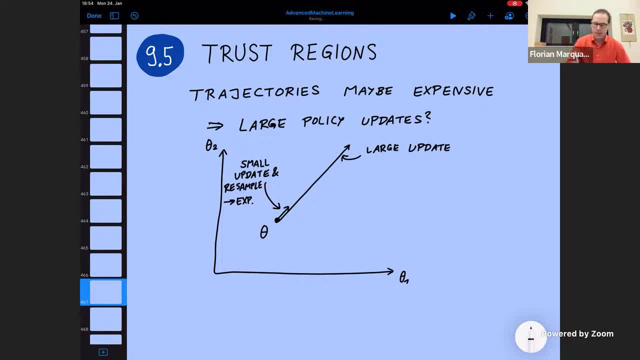 if you take steps that are that large, So it's unreliable, So it's unreliable. You can also try to say: let me keep whatever information I have and which is contained in the current value, function and in the states and actions that I have observed, but let 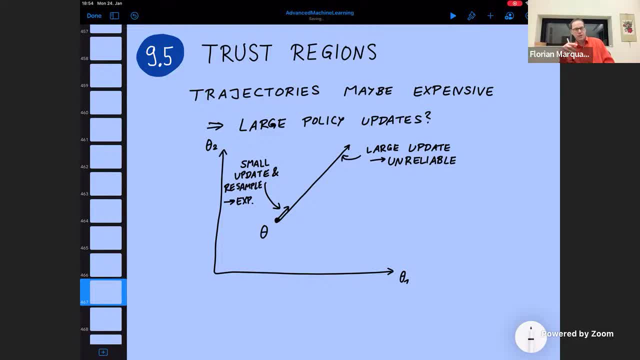 me still do several steps in the gradient update of my policy. so it could look like this: So the value function is not updated, but you take multiple gradient steps with respect to your policy. But the question again is when to stop, because eventually this will no longer be good. 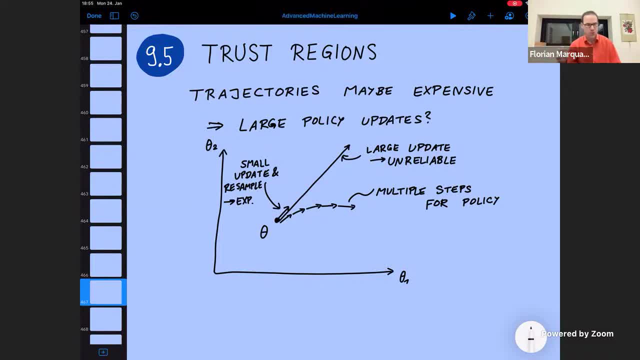 The value function should have changed your policy. It's now different. So what to do? So the question is when to stop with this procedure, And so you could say: well, I say that theta should not change by more than something. So you could put a bound on theta or the change. 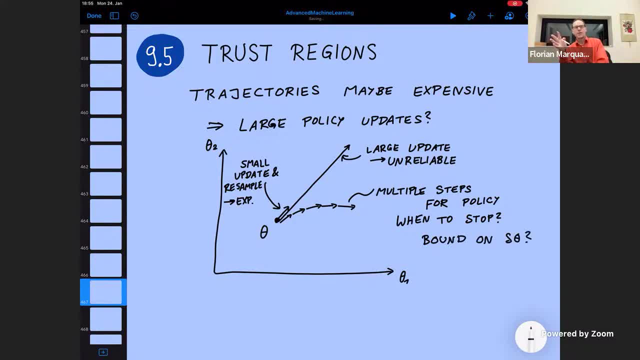 But then you say: how do I know what is even the meaning of these parameters? These are just weights and biases in a neural network. There are thousands of them. Their meaning with respect to the actual dynamics that the policy encodes can be very different. 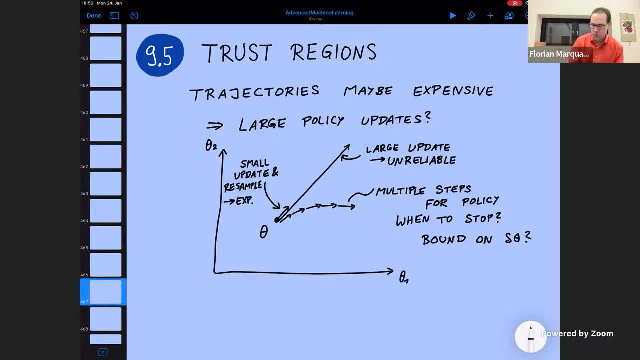 depending on the network structure and everything. So that's why you slowly kind of come up with the idea that maybe you should put a bound on something else, and the something else could be the policy. So the change in the policy maybe should be bounded. 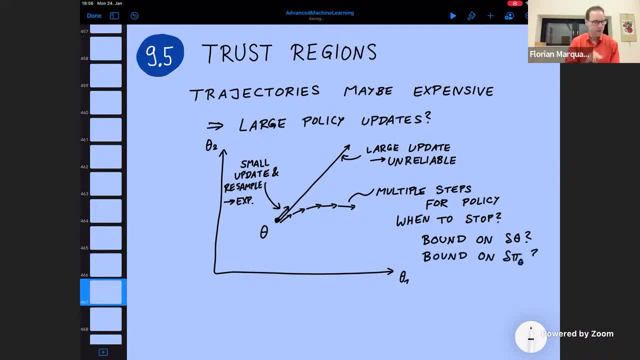 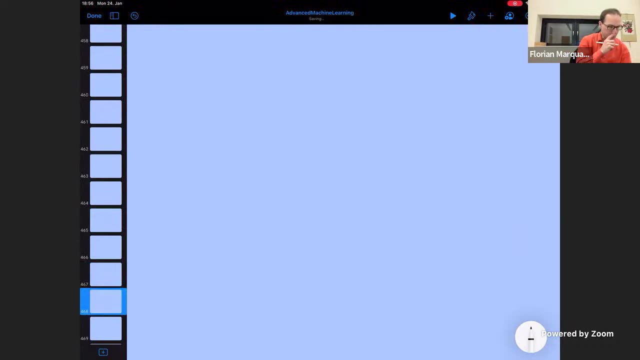 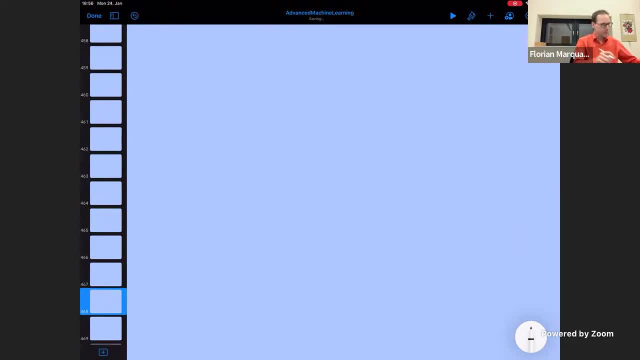 But now let's start the actual story. Let's have a look again once more at the formula that we need for our policy update. So that was the advantage times, the gradient, And now I'm going to become a little bit lazy. I'm dropping many of the subscripts and so on. For example, the time index is no longer there. 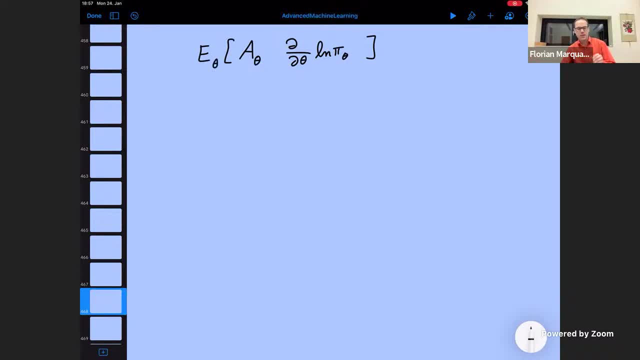 because I really want to focus on the parameters theta. So when I write e theta, what I mean is I take an expectation value with regard to the policy encoded by theta, by the parameter theta. So all the probabilities and so on, they are calculated according to theta. When I write a 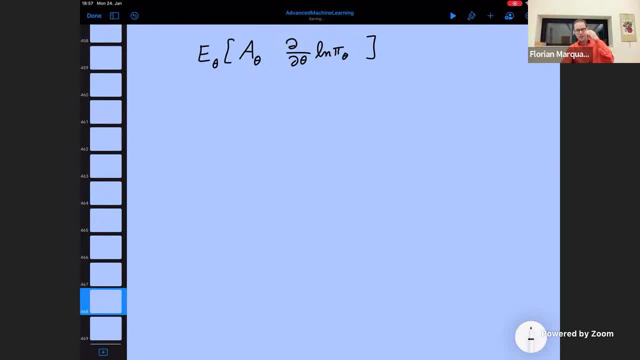 theta. I just mean that this is the advantage that is calculated according to the value function for this particular policy: theta. And again here theta appears. Okay, Now we of course remember, just to make it clear, That both of these parts depend on the state and the action. 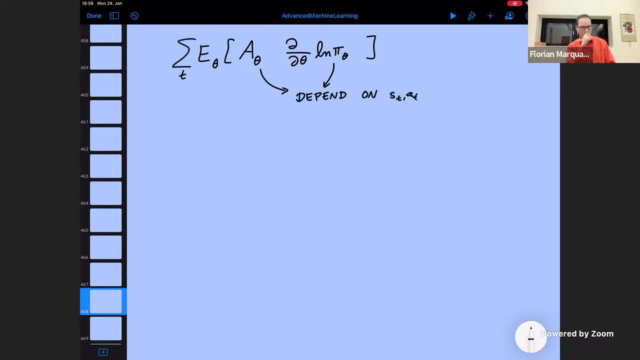 And also we remember that eventually we will sum this over all time steps. Okay, So this is where we start, And now let's do something funny. Let's take the logarithmic gradient and do a step which is, so to speak, backwards of what we had done initially when introducing this logarithm here. 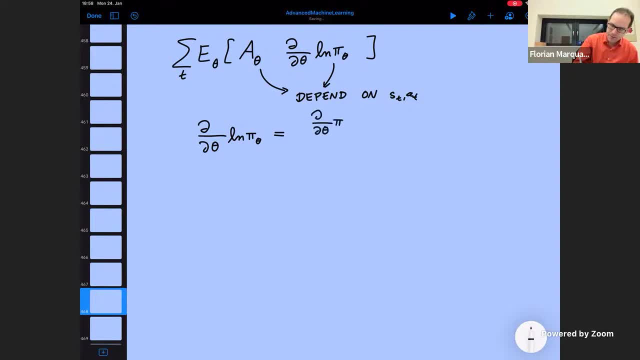 Because we could say: well, according to the elementary rules of taking gradients, this is the gradient of pi divided by pi. So that's correct. And so now you realize that if you write it like this, the formula written up here would appear in another maximization problem. 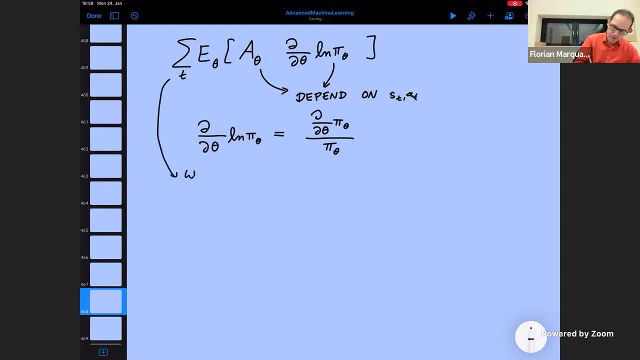 Let me show you something nice which is pretty cool, so that you can actually do in the moment they are being calculated. So let's start here. So you see, this is going to be the point where we have discriminant based down So we can600 Wars. so play along the first line. we know which output L is. 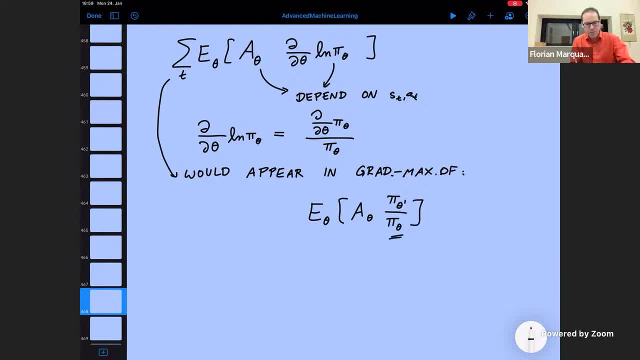 So what is L? And let's take B And again that aos three to the essere factor over the other power. I just have pi theta, but in the numerator I now have pi theta prime. Theta prime will be what we will optimize over. 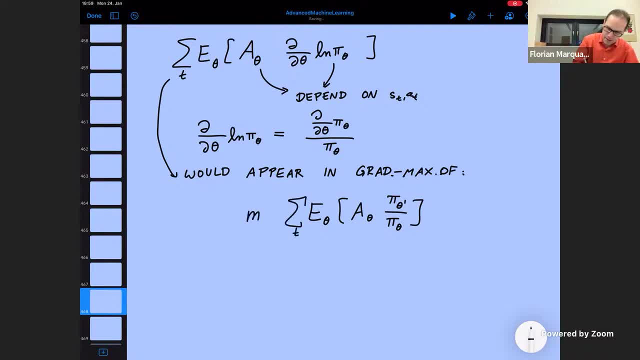 So if I now have the summation and then I say I want to maximize this over theta prime and I want to do it using gradient ascent, and I start with theta prime equals theta, then of course the gradient written up there would be what appears in the first step. 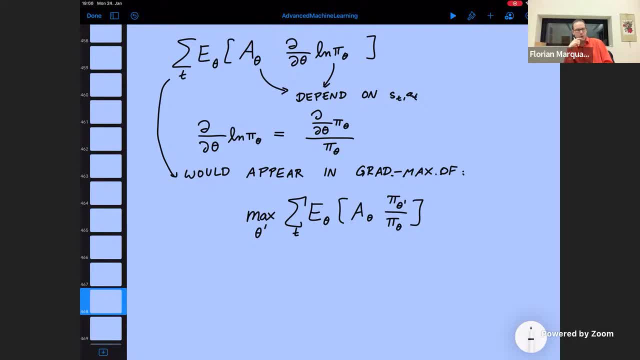 And so the hope, or the naive hope now would be to say: well, let's just do this, Let's just, instead of only taking one gradient step, literally maximize the quantity down below with a sequence of gradient steps with respect to theta prime. 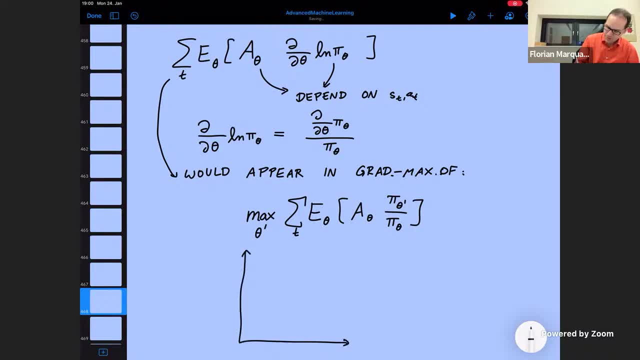 So the graphical version of this would look like this. Here's now theta prime space. I start with theta- prime equals theta initially, And I want to do several update steps of gradient ascent of this new formula where, remarkably, the advantage function is kept fixed. 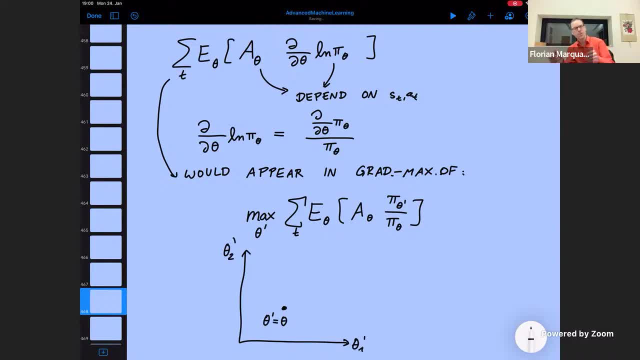 Also, this expectation value is still with respect to the old fixed policies, So the states and actions you have are run according to the old probabilities. But the thing that can change is here in the numerator, the policy. And so if I do this, 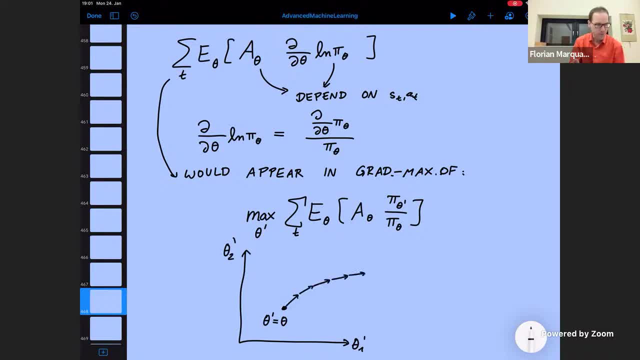 I can get some interesting flow in theta prime space and then maybe I end up maximizing this. So that would be the trajectory if I try naively to do this Now. again the question arises: is this all reliable? And certainly it will no longer be reliable. 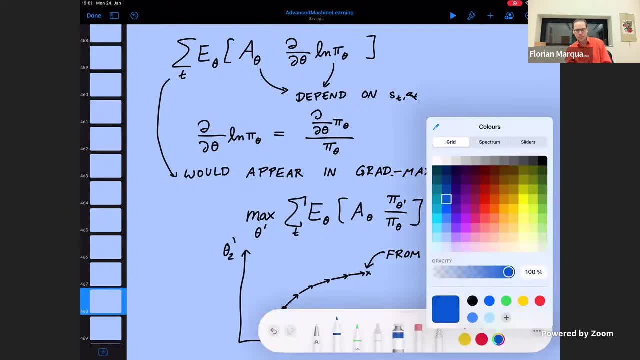 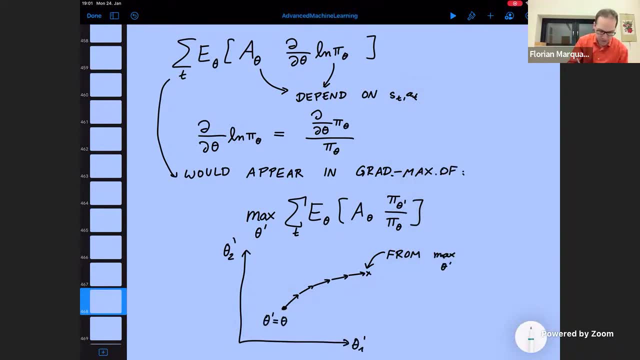 if I go too far from the initial position. So what will happen is that the correct flow of theta prime may be different. They might coincide initially, but if you deviate too far it's no longer good. Okay, So again there comes the question. 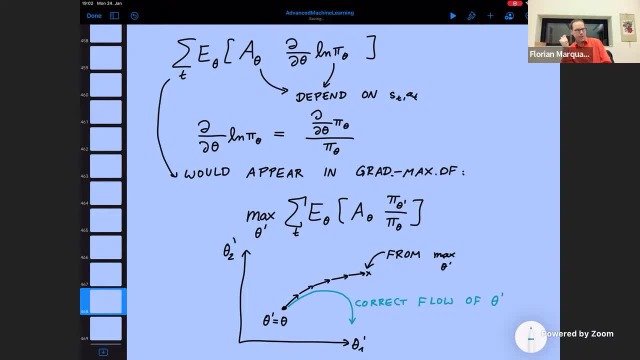 how do we limit the amount of change in theta? And I already indicated that it's smarter not to look at theta- how much theta changes, but it's smarter to look at how much the policy changes, because that's what matters in the probabilities. 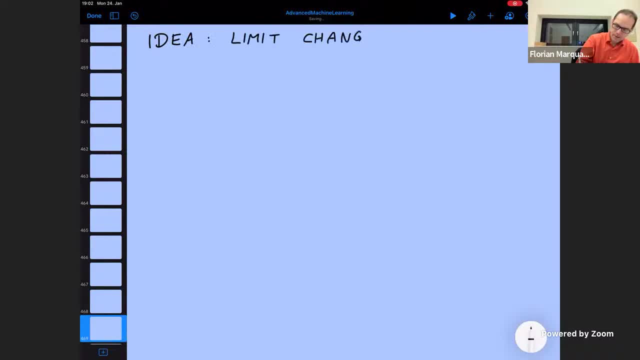 So we want to limit the change in the probabilities. Now, obviously, to limit the change, you want to say something like the old probabilities minus the new probabilities. somehow that should remain small. But we know already how such things are done. Namely, you compare two probability distributions. 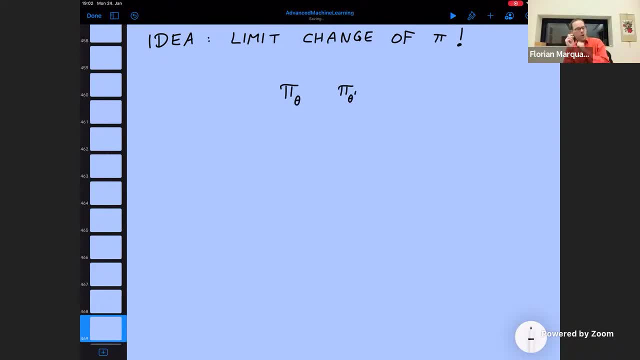 by using the probability distribution. So if you look at the probability distribution, you can see that the probability distribution is smaller. Okay, So this is the Kullberg-Leibler divergence, And so you would then say this should remain smaller than some reasonable threshold delta. 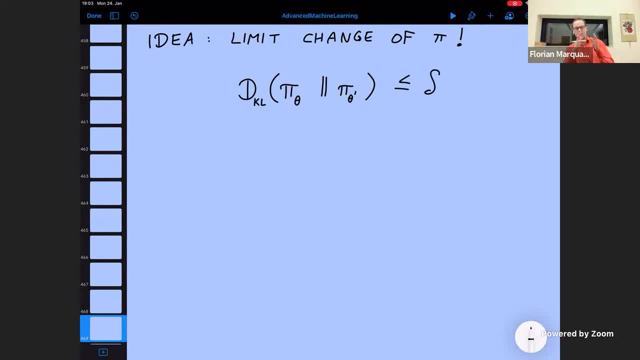 And so this delta should typically be smaller than one. of course, imagine, these are action probabilities, So it's a discrete set of actions, And you want, say, delta to be smaller than 0.1 or something like this. And just to remind everyone, this is the expectation. 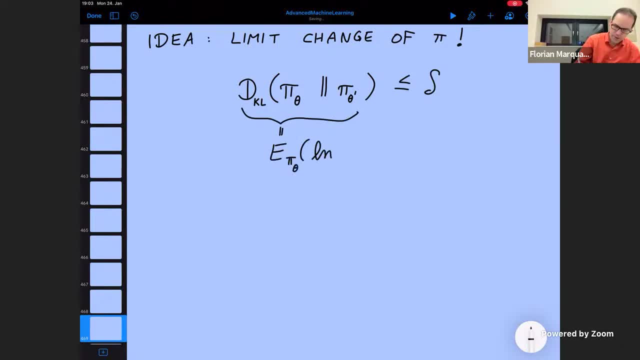 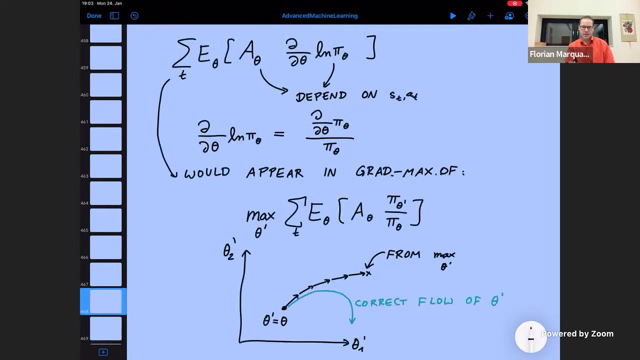 This is the expectation value with respect to pi theta. That is the old policy of this, of this ratio. Okay, And so this whole strategy of saying let me maximize this quantity here, but let me not get too far with respect to my policy, 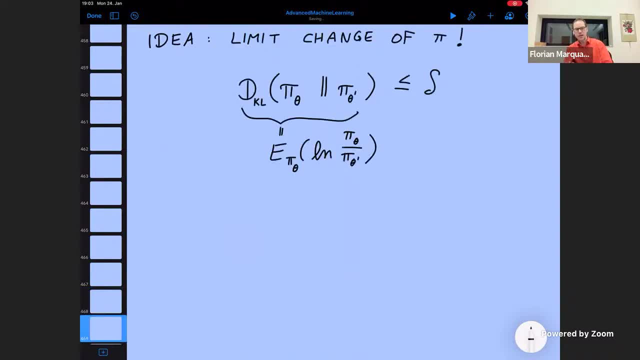 and keep the- let me maximize this quantity here, but let me not get too far with respect to my policy- and keep the and keep the, the Kullberg-Leibler divergence constraint. This whole idea is called trust. region policy optimization. 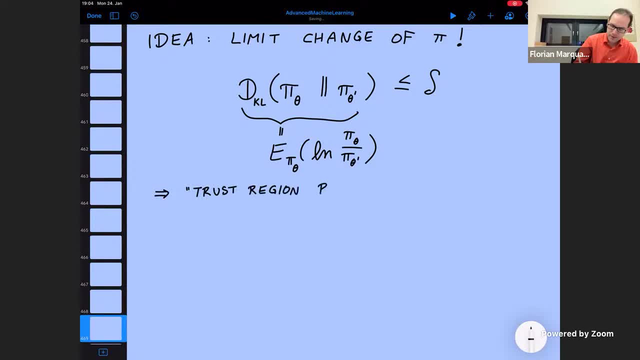 And now you understand why it's called like that: because the trust region obviously means you are trusting the whole scheme only within a certain region around your own policy. Okay, So that was introduced, I believe, in 2017.. So that's now a few years old. 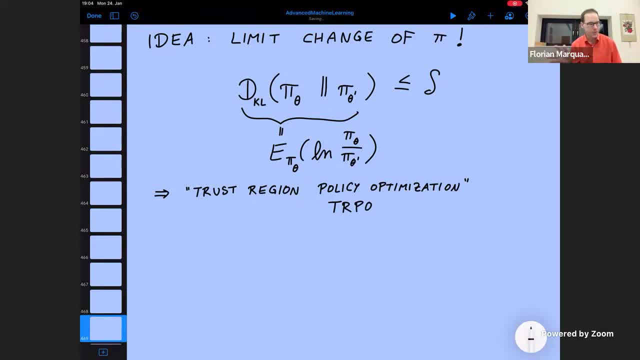 It's not yet the complete state of the art, but we're getting there. Now the question is what to do about the Kullberg-Leibler divergence, And one idea you can have is: let you say: well, let me just do a quadratic approximation. 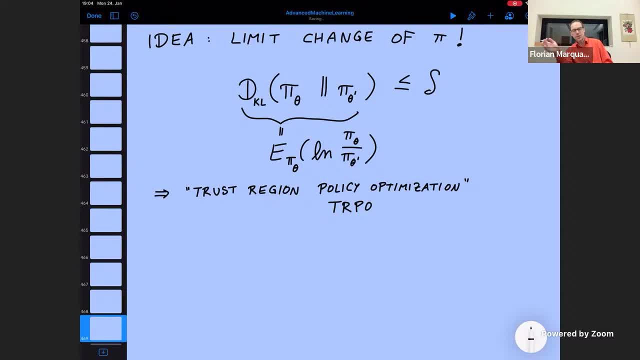 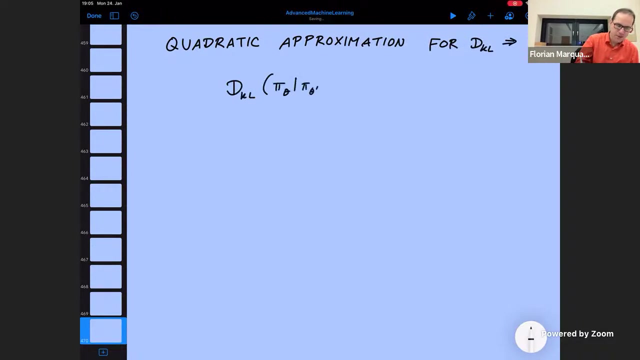 since I'm not going very far anyway, let me do a quadratic approximation. Okay, quadratic and the shift of theta, and so if you do that, you recover something that we have discussed before. if someone takes a Kullback-Leibler divergence between two relatively close by probability distributions that are parametrized, 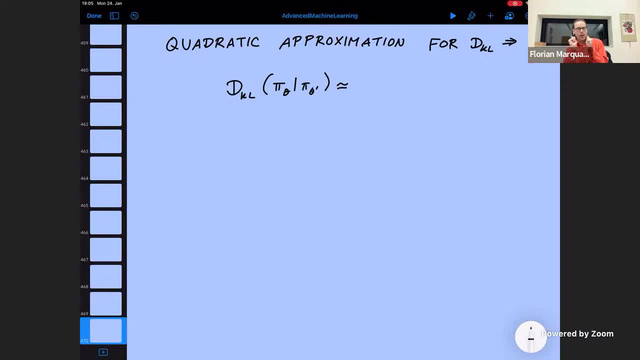 so you shift the parameter a little bit and you do the quadratic approximation in the shift, you end up with a term that involves the fischer information matrix. so you get something like this: that's the difference, that's the fischer information matrix, and again the difference. 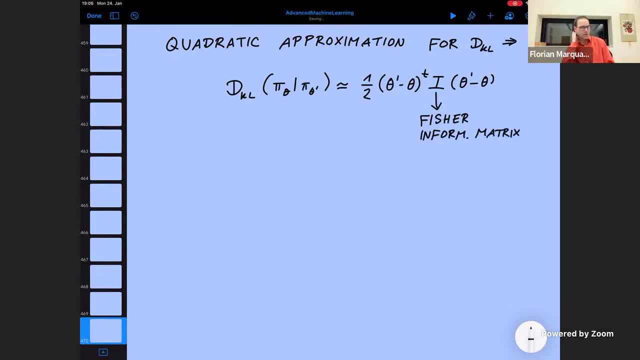 so to speak. the fischer information matrix is like the curvature of Kullback-Leibler, and so if you now try to maximize, in the sense that you want to keep this quadratic approximation to Kullback-Leibler within some maximum value, then how does? 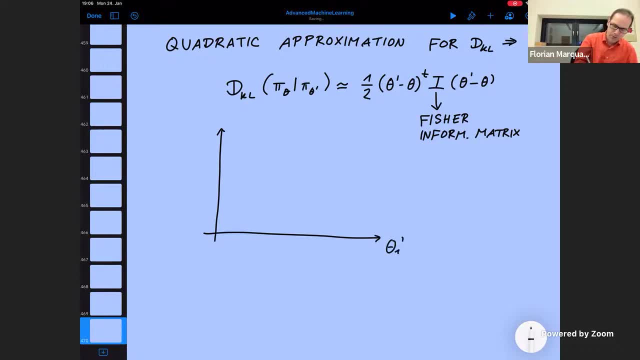 it look like it has a very nice geometric interpretation which you will recognize in a moment, probably. so here we are. theta is our current parameter. we want to move away from theta in order to optimize our expected advantage times, the ratio of polices. so we want to optimize this term. 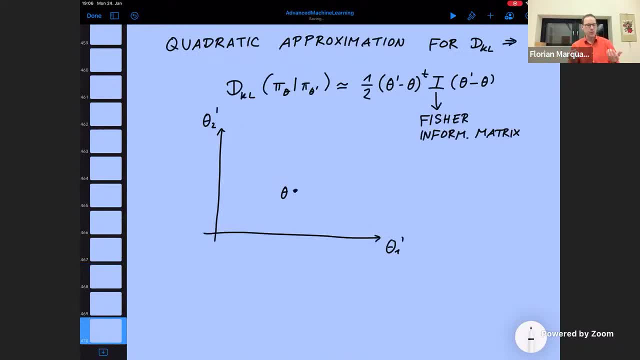 but we want, don't want, to overshoot, so we want to keep the Kullback-Leibler confined. So I can draw the region in which Kullberg-Leibler, according to this quadratic approximation, is smaller than or equal my little delta. And it turns out, since this is a quadratic approximation, 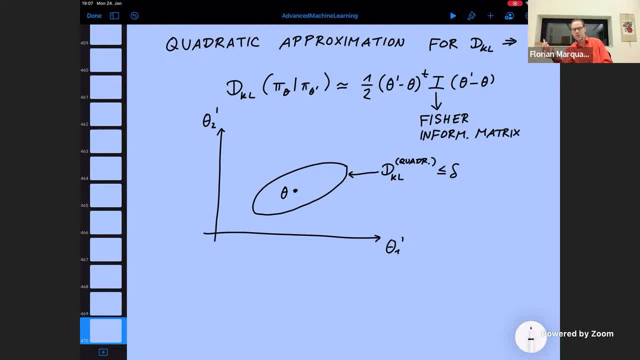 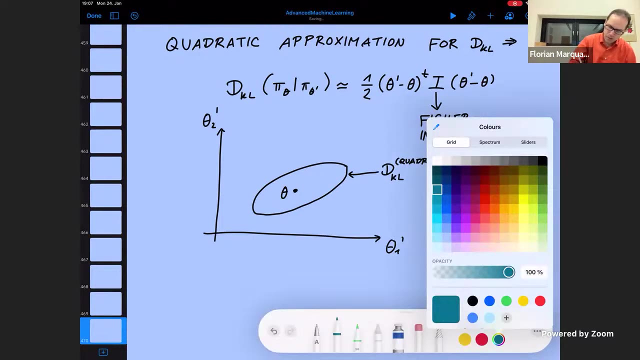 you find some ellipse or some ellipsoid in higher dimensional spaces. So this is all the region I'm trusting, And then we can come back to two old friends. So there would be now the naive gradient of what you're trying to optimize. But if you go, 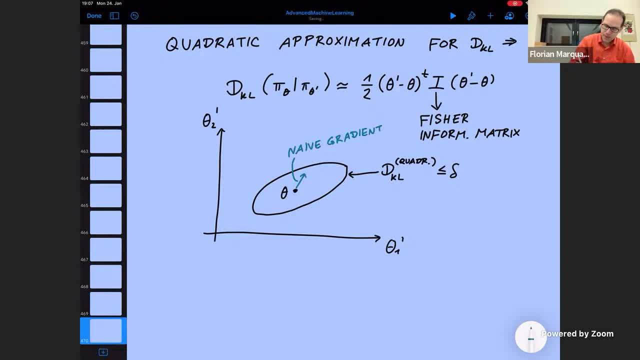 And if you go and really optimize with this constraint, then you might end up in a different spot. Also make a bigger step maybe. And this is just the natural gradient. So at least if delta becomes very small, then this is exactly the natural gradient. 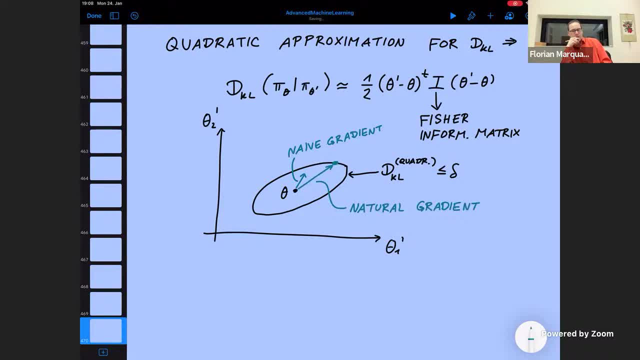 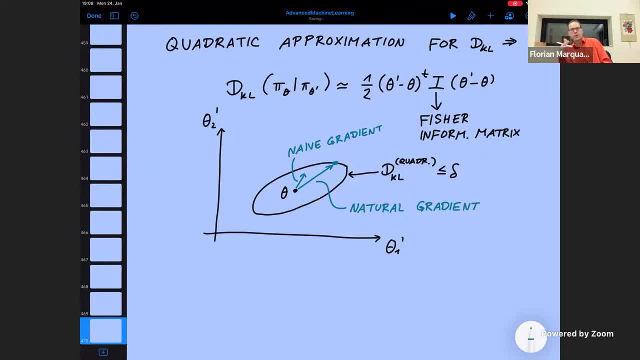 Still, if we do this quadratic approximation, we do need the Fisher information matrix And that is expensive. So we want to have something better. So that was one idea to stop and say I have all of my states and my actions and I have updated my value function. 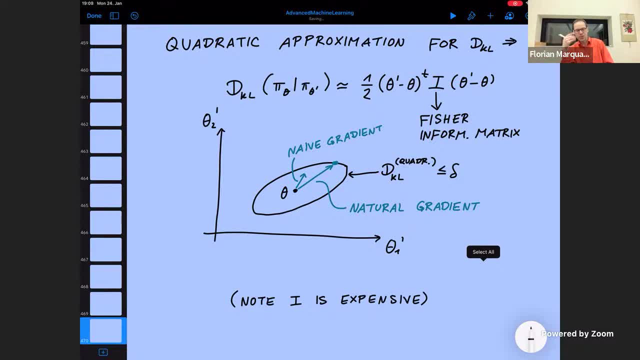 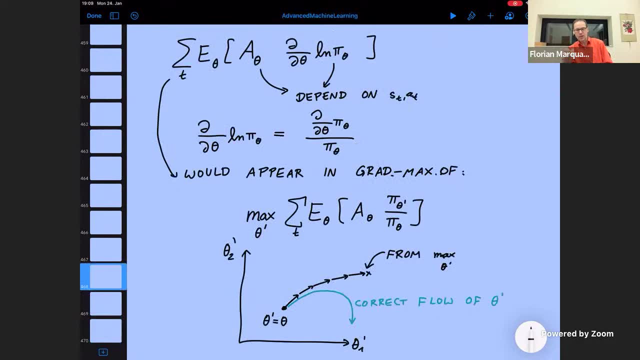 And now I don't want to play new trajectories, I just want to do a little bit more carefully my theta update with respect to the policy, And so one ends up maximizing this thing, but one doesn't want to overshoot because it's dangerous. 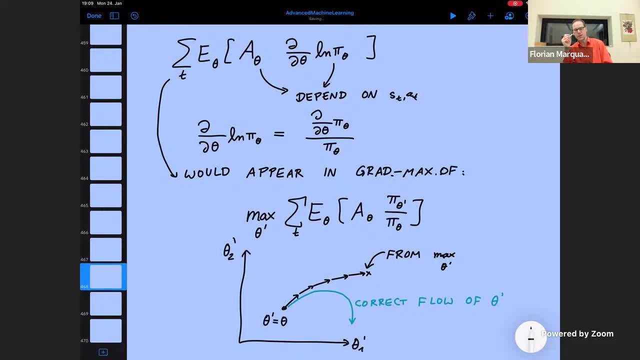 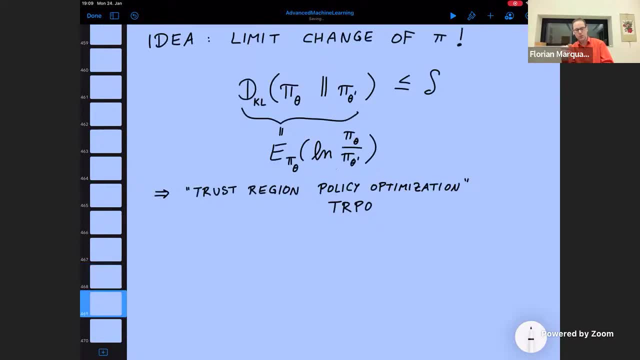 Then maybe something bad happens to the ratio there of policies, And so what one does is one restrains the total amount of change, which one can do using the Kuhlbach-Leibler. One can do quadratic approximation. that leads to the Fisher information matrix. 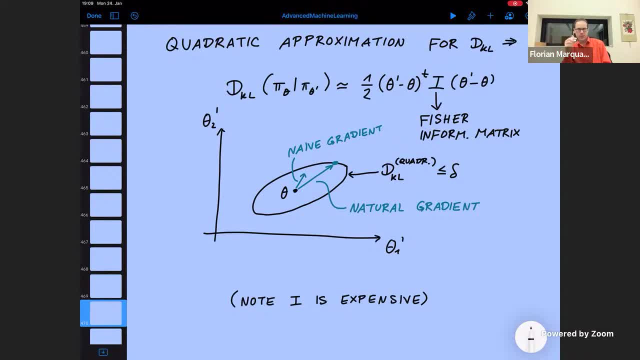 And then you get what we described here. Okay, so that is still not quite state of the art. because it's still not quite state of the art, It's still a little bit more expensive than you actually want it to be, especially this quadratic approximation. 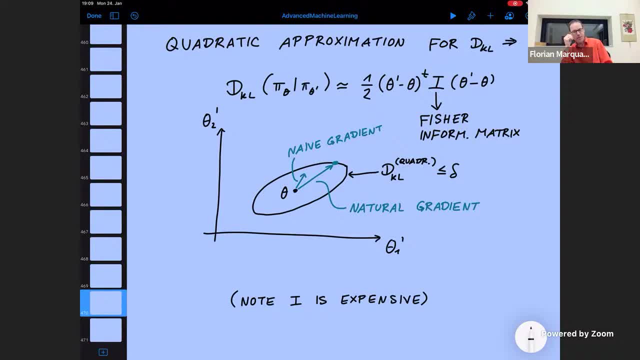 You need the full Fisher information matrix. So then people came up with another idea. They said, well, instead of doing this quadratic approximation, why not take the Kuhlbach-Leibler series and just do also gradient ascend with respect to the Kuhlbach-Leibler term? 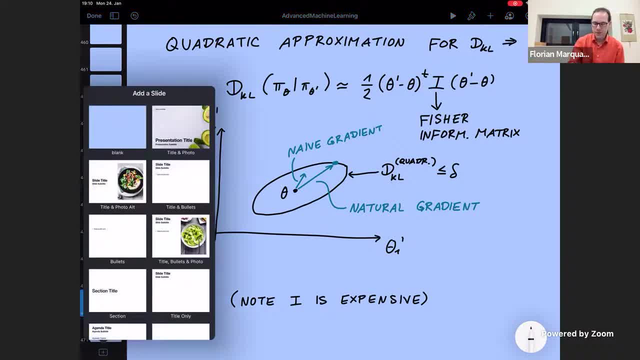 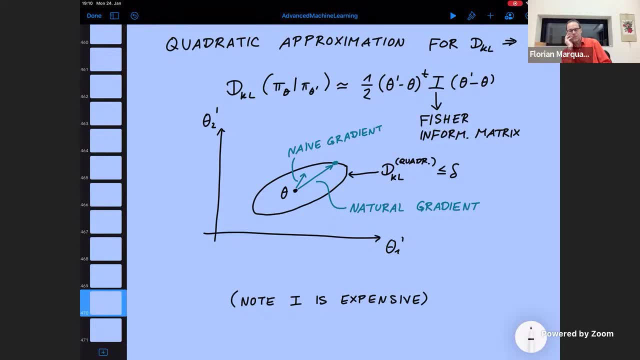 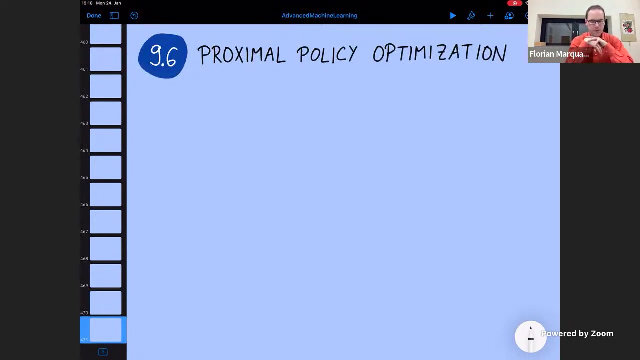 So let's see how that works, But first again I should ask: is there, is there some question here? Okay, so not for the moment. Let me then move on. And this is not really the state of the art method that we are using all the time in our research. 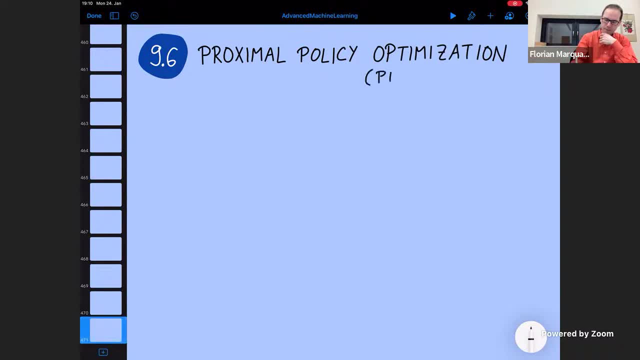 It's called a proximal policy optimization And, again, literature references will be on the website. Now, how does this work? So it is from the same authors as TRPO, So it borrows many ideas, but we want to do without this. Fisher information matrix. 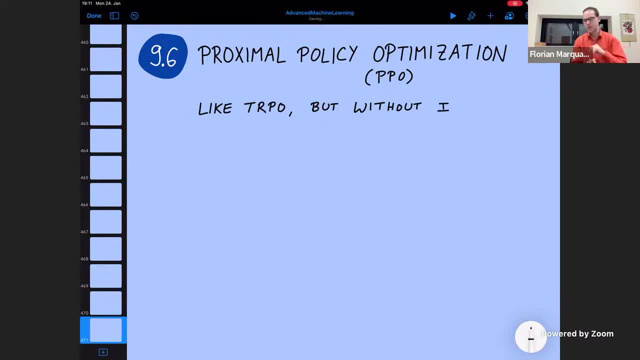 So how to do that? So there are two options, and I will first tell you the first option that still has the Kuhlbach-Leibler divergence, but then there's a second option that is even easier. Still, it's good to start with the first option. 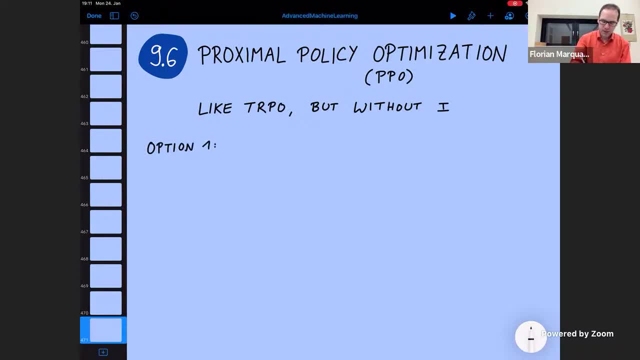 So let's see, we could have this quantity that we're trying to optimize and then we don't want to overshoot. So we could have this hard constraint that we were talking about a moment ago, where we say the Kuhlbach-Leibler is constrained. 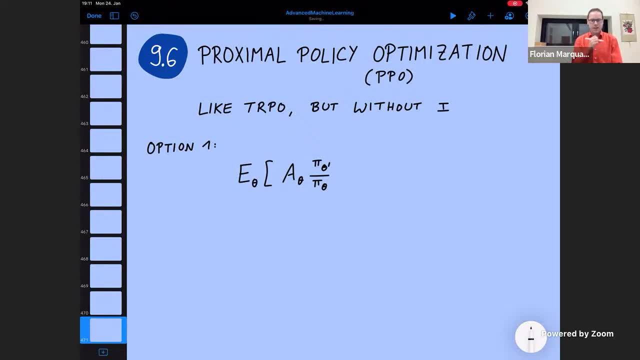 up to some delta and cannot be larger than that. but we could have this constraint up to some delta and cannot be larger than that. cannot be larger than that, but we can also do it in a more soft way. So this will try to become as large as possible. 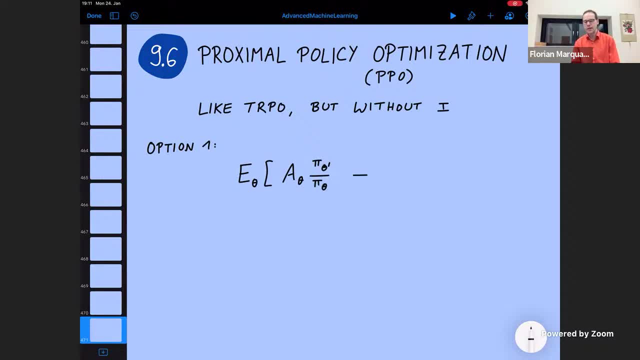 So if I subtract something that is proportional to Kullback-Leibler, then this will counteract it, because eventually that will also become large and then I don't win overall. So that's the idea here: in a soft constraint So I have Kullback-Leibler. 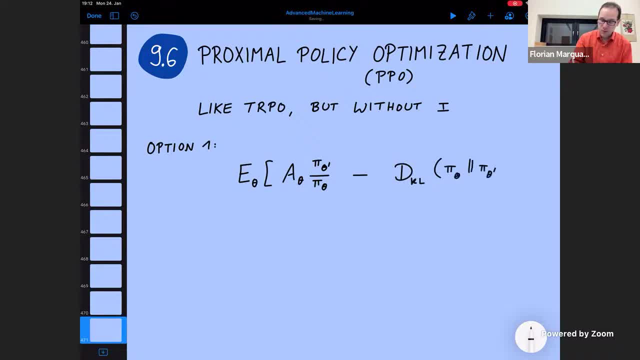 with some pre-effect term. let's call it beta, And then I want to maximize this. Obviously, beta is like a Lagrange multiplier, yeah. So if you wanted to do constraint optimizations such that eventually, the Kullback-Leibler is equal to some value, 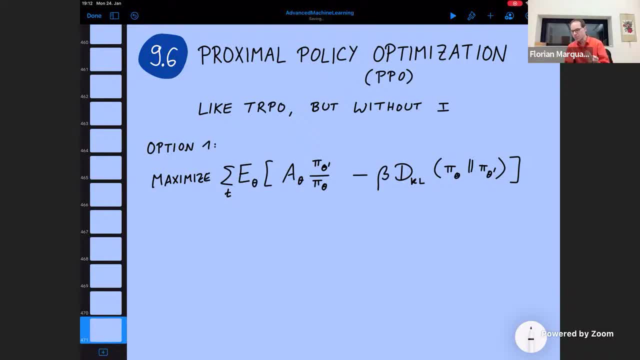 then you would need to solve this optimization problem for an arbitrary, arbitrary beta and then later change the beta until you hit the right value with your Kullback-Leibler. That would be a little bit too expensive. So they have a smarter approach. 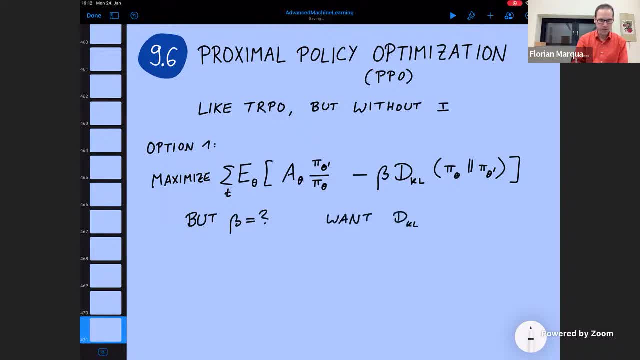 So remember, we want that eventually the Kullback-Leibler will be smaller than or on the order of delta, And so the idea is to adapt beta, If you look at it closely. I don't even write down the steps now. 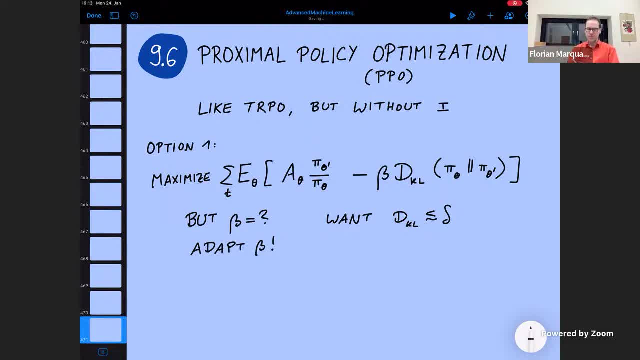 but I will tell you in words, because then we move to the other scheme. that is even better. So let's say, if beta is very large, then that means this Kullback-Leibler term has a big influence, which means you don't get very far. 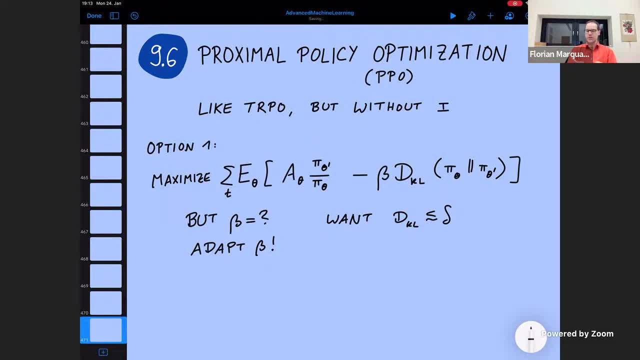 because otherwise the Kullback-Leibler will become too large. And then this term hurts you because it's coming with the negative signs. So if beta is large, the resulting Kullback-Leibler divergence will be fairly small. Now if it is much too small. 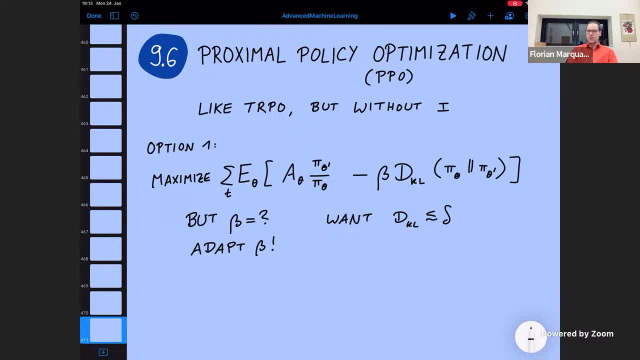 much smaller than delta and you observe this, then you can relax the constraint. Then you just choose beta a little bit smaller for the next step of your gradient ascent And then the constraint will be relaxed And, as a consequence, the Kullback-Leibler divergence will tend to increase. 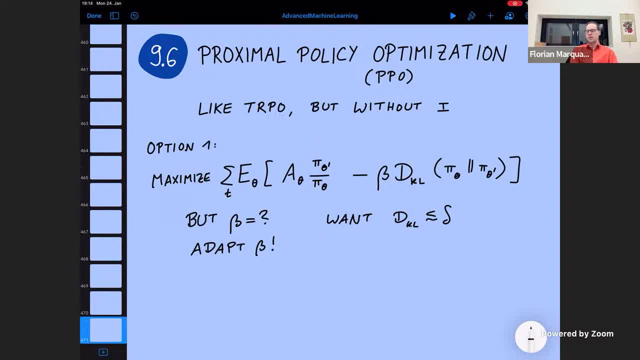 On the other hand, if you overshoot, if the Kullback-Leibler divergence turns out to be really large, much larger than delta, then what you do is you, you must tighten the constraint, So you must make beta larger again. 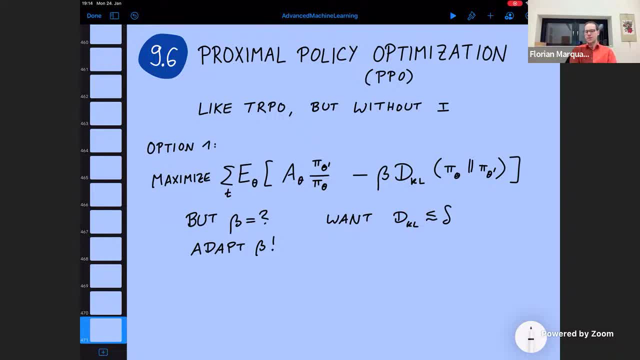 in order to push down the value of the Kullback-Leibler divergence, And so this is what goes on in this scheme. So you do multiple gradient descent steps on this cost function with respect to theta prime for some fixed beta, And then you check what happened. 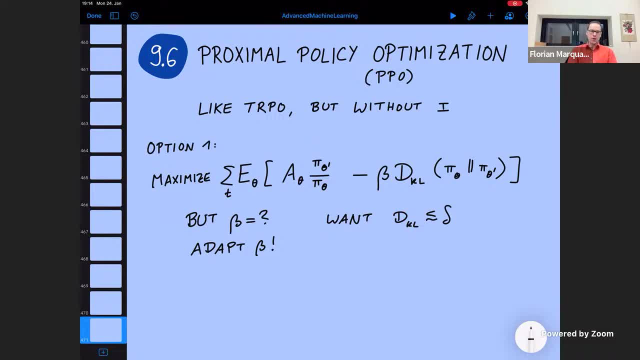 with the Kullback-Leibler divergence- Is it too large or too small? And depending on that, you adapt the value of beta In order to calibrate it to go to the kind of data that you wanted. So your steps will neither be too small nor be too large. 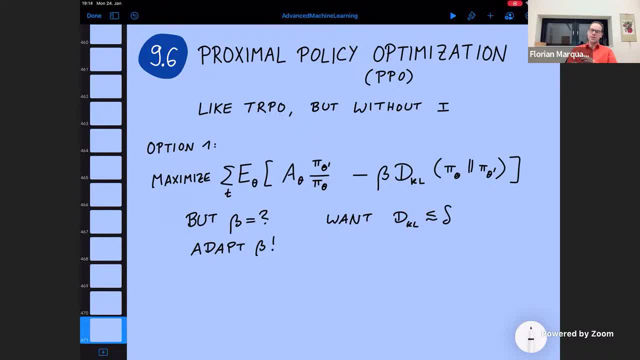 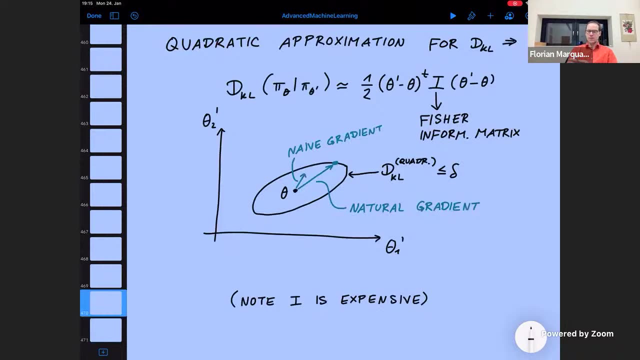 And since everything is done in terms of gradient descent, you never really need to do this quadratic approximation for the Fisher information. Now, whether I should say whether this is actually expensive or not, it depends a little bit on the number of parameters you have. 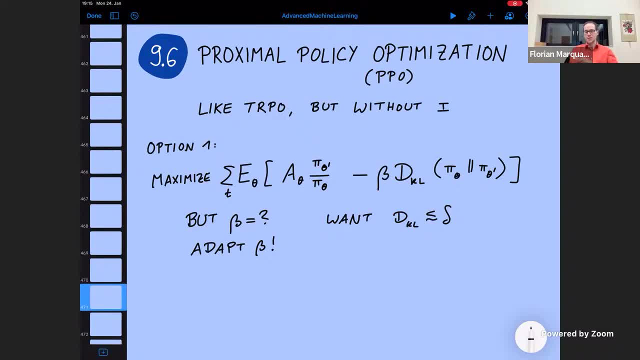 But if you have a neural network you can do that. If you have a neural network, then theta is of course all the weights and biases, So it can be quite expensive, Okay, so that is option number one and it works. It works nicely. 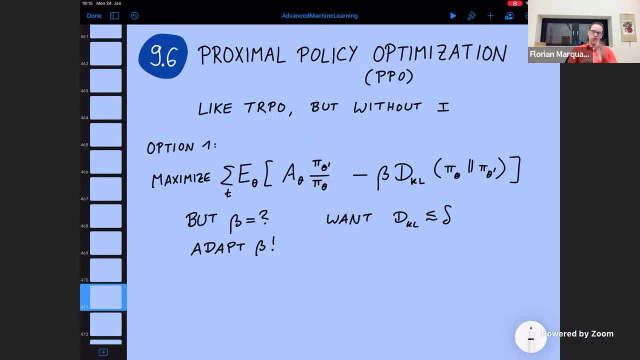 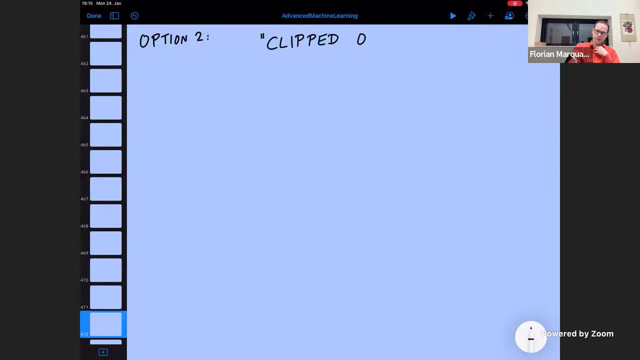 But there is another option, which is even cheaper in a way, And so this is what everyone uses, And so this comes by a name. it's called clipped objective, And so that's the preferred scheme nowadays. So what's the idea? 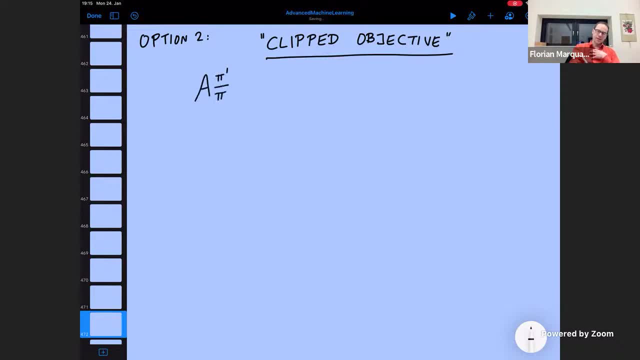 Essentially, we're trying to optimize something like this. Now my notation, you'll realize, becomes more and more bare bones. So it's the advantage times, the new policy divided by the old policy. Now, of course, if the new policy 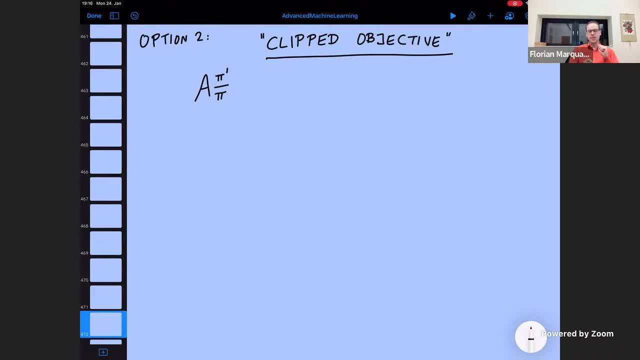 say: the advantage is positive, then it's good, But if the advantage is negative, then it's good. But if the new policy is positive for some action, if the new policy for this particular action becomes larger and larger and larger, this seems better and better and better. 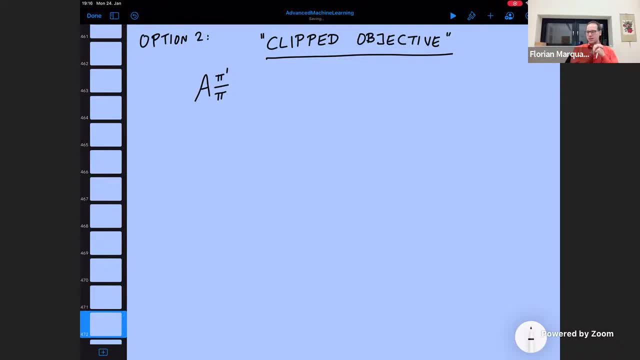 And at some point we need to stop using this, say, Kullback-Leibler divergence. But there's another very easy way to stop this runaway effect when you want to make the policy pi prime ever larger and larger, And that is simply if you arrange things such that. 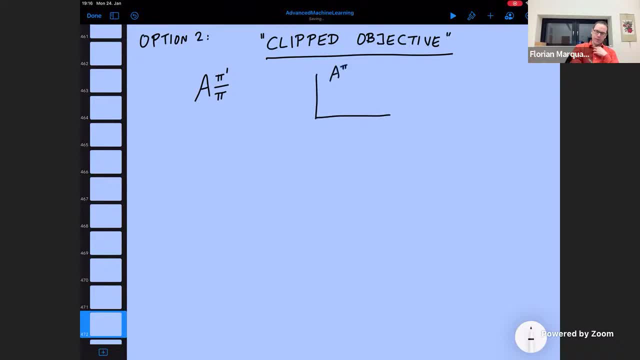 a pi. well, that your objective. so let's call this the objective And let's plot here something like pi prime divided by pi, say, for a given action, And let's see, instead of having just a runaway effect, where this becomes ever larger. 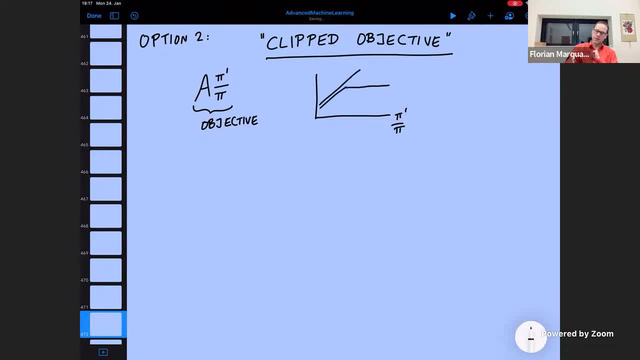 you want to arrange things such that it doesn't become ever larger, So this is a modified objective, so to speak. If you do it like this, then there is really no incentive to go to very large values of this ratio. So how do people do this? 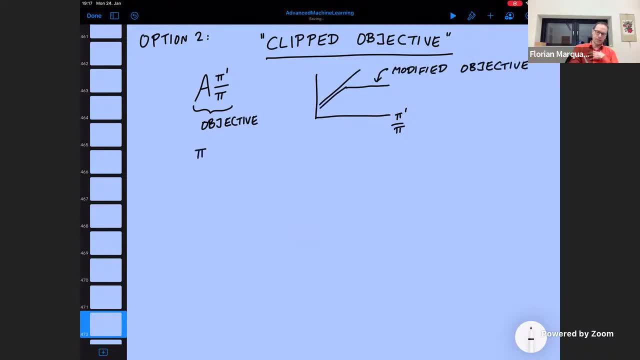 Well, there's a very interesting and simple technique: Instead of directly taking this ratio, which can become ever larger, you just replace it by something that is, so to speak, clipped, so which only is in a range, a range of values. 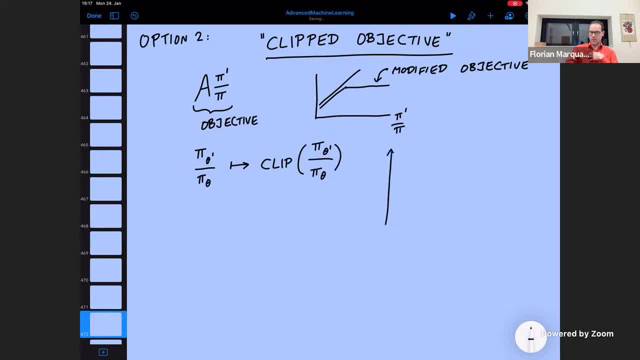 So how does this look like when we clip things? Well, so again. so now a little bit more carefully, I'm plotting the pi prime over pi, say, for a given state and a given action, And now I start of course at one. 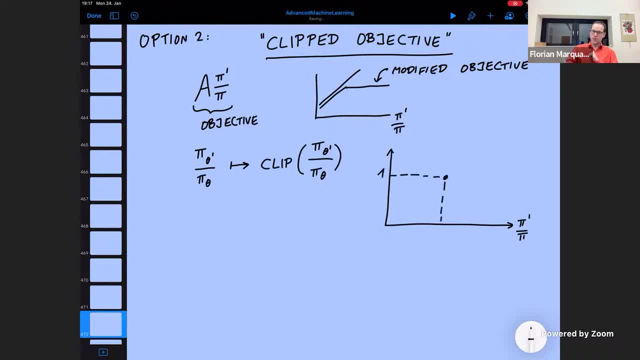 One is the special value when the new policy and the old policy coincide for this action. And now I in principle go up when I increase pi prime over pi, But at some point I want to clip it Instead of going further up. I just say that's it. 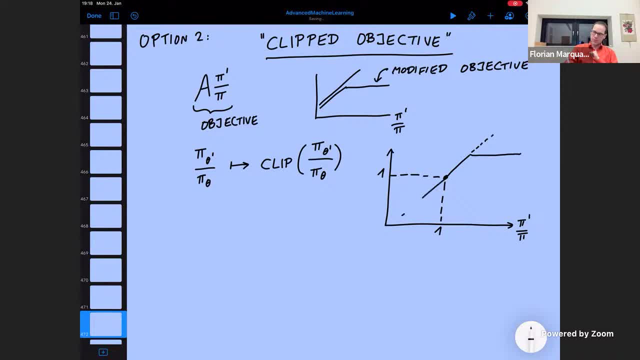 I can also go down And again at some point I stop and I say: that's it, And I can do this in some range. So let's say, that's maximum one plus epsilon and minimum one minus epsilon, And I choose the epsilon myself. 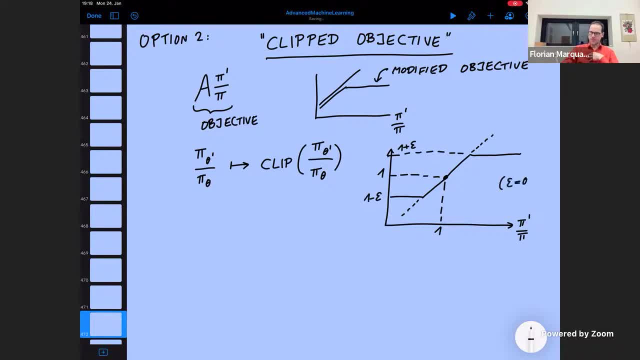 Typical value is that people use is 0.2.. Okay, So I make sure that I never go too far. Okay, So I make sure that I never go too far far, and there then is no real incentive to go very far away because your objective no. 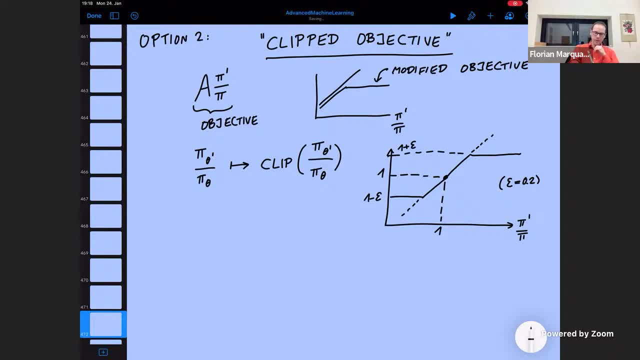 longer increases. There is still a catch, and the catch is the following: You might have a situation where one action is bad, so say the advantage is negative, Other actions are good. You are trying to push up the policy, the probability for the good actions. 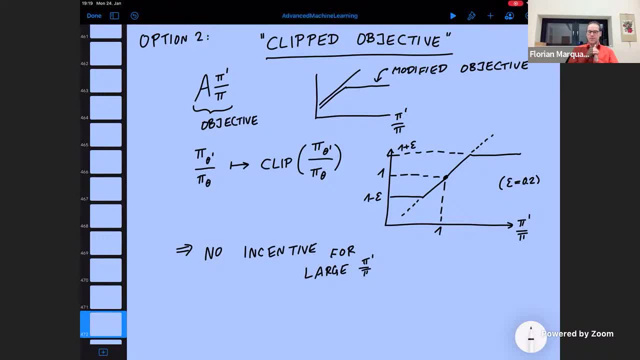 You are reducing very much the probability for the good actions. Let me see how this goes. There can be cases so I have to start again. There can be cases where this estimate that you would be doing here if you just have the product of the advantage and this clipped ratio, is still too optimistic because maybe 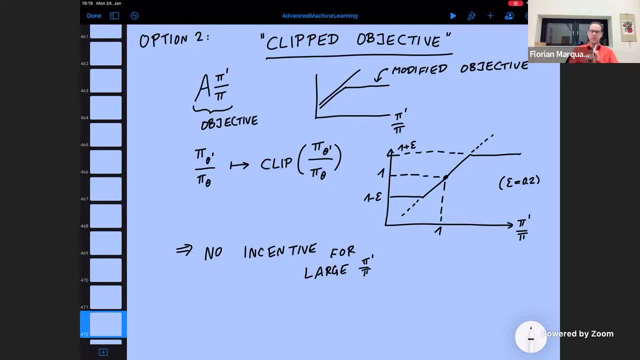 something was already clipped. that gets multiplied by a negative advantage, so it seems as if things are not that bad, but in fact they are really bad. so you need to make sure that you always take the most pessimistic estimate, and so what people introduce them as the rule in total is to replace the original objective. 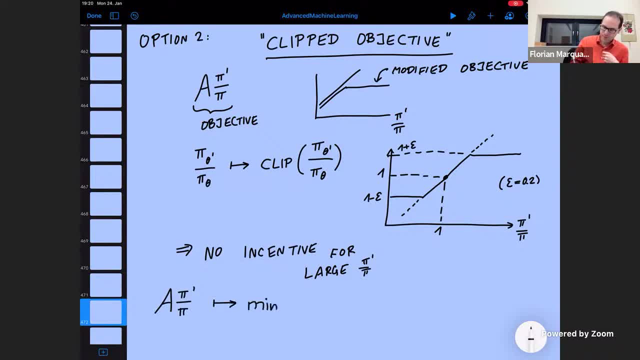 by the following: you take the minimum of the version where you clip it and the original version, so that guarantees that your estimates are always as pessimistic as possible. so you don't do anything stupid. maybe you could have gotten a little bit better, but it's good to be on the safe side, and so this is it. you take the advantage. actor critic. 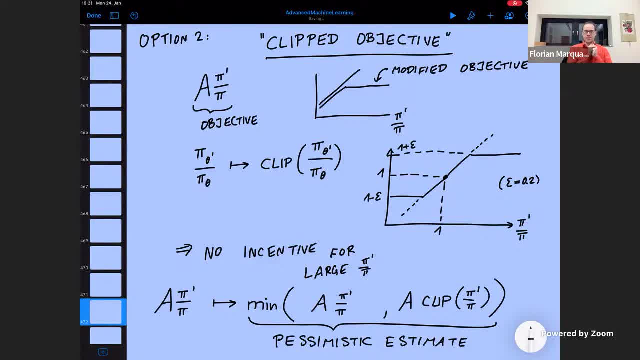 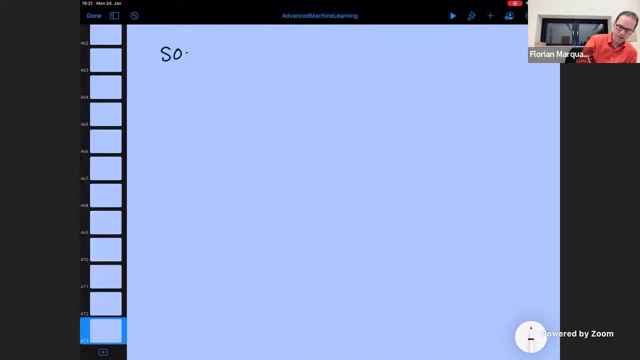 scheme that we have discussed before, and you just replace the advantage times, this logarithm of the policy you explain, replace this by the formula shown here. so, to summarize, we would have had, in this cost function that i showed a few slides ago here, in this cost function that we are trying to optimize, we would have had the advantage times. 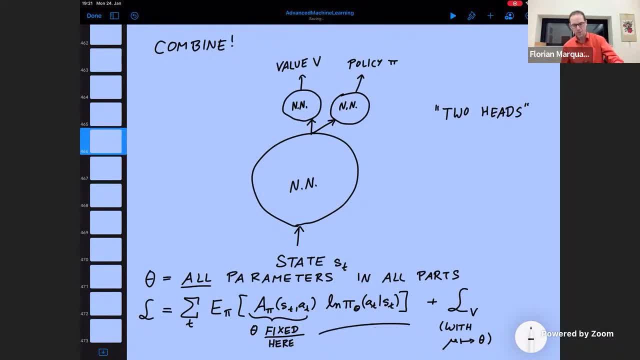 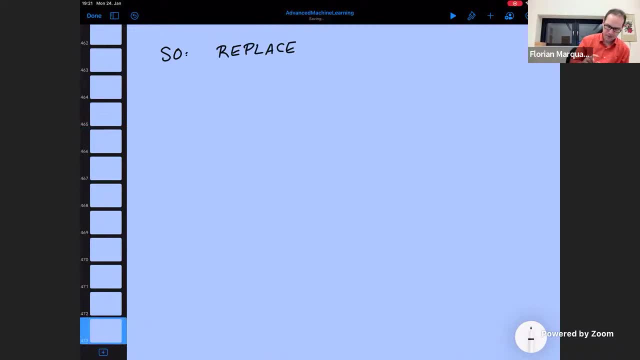 logarithm of the policy and we replace this part by this clipped objective. so this is the cost function. so a times log of the policy by a- sorry, by whatever we wrote up here. so the minimum times, the, this one. okay, so that seems a very simplistic scheme of doing things. it is very simple and it works very well. 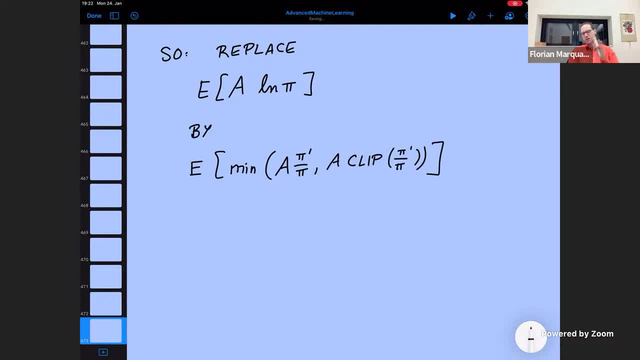 and so it has found really widespread use, and that's the standard technique. if you don't know anything else of how to, how to approach a deep reinforcement learning. this is what people do nowadays, so this is the ppo method. no kolbach leibler is needed. 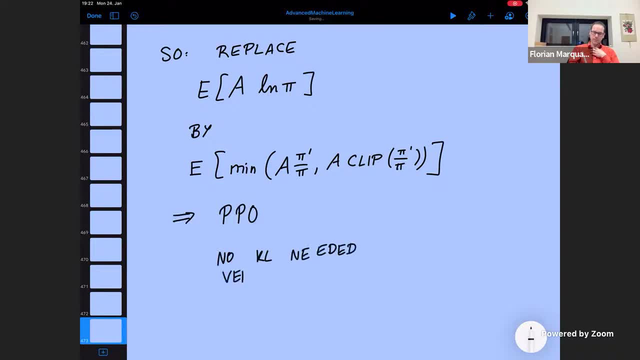 it's very simple and it works very well. okay, now you can, of course, try to implement it yourself, and it's entirely possible, and let's see whether we will do a little exercise. but then again, there are many little tricks and parameters here and there, and so these days, 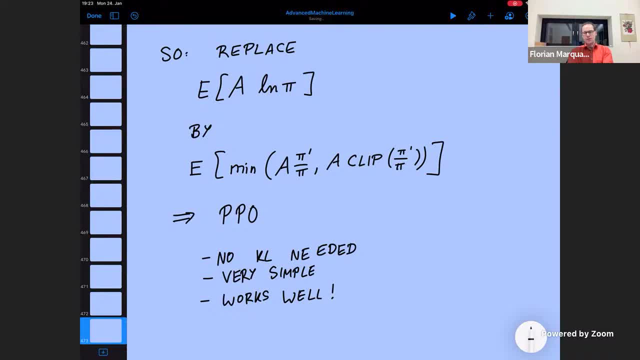 there are very good frameworks for doing reinforcement learning. so there is one framework by google and one framework by open ai and probably several others which i don't even know about. so whichever taste you have in terms of reinforcement learning or also in terms of deep learning, whether you're using tensorflow or pytorch- 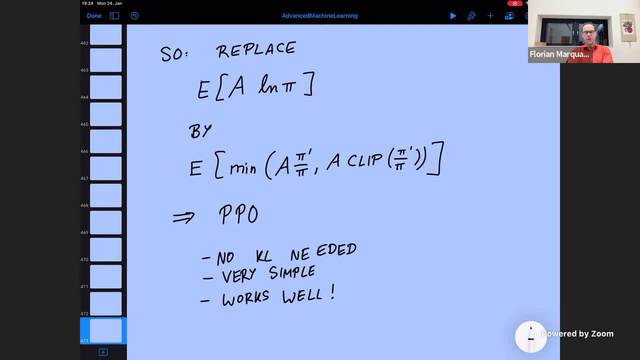 you will probably find a good reinforcement learning framework, and ppo will always be there as one default option. okay, very good, so any questions and other questions? okay, so i don't see any further questions, so it's probably better to stop at this point for today. next time we will go on and say a little bit about continuous actions, because right now we always 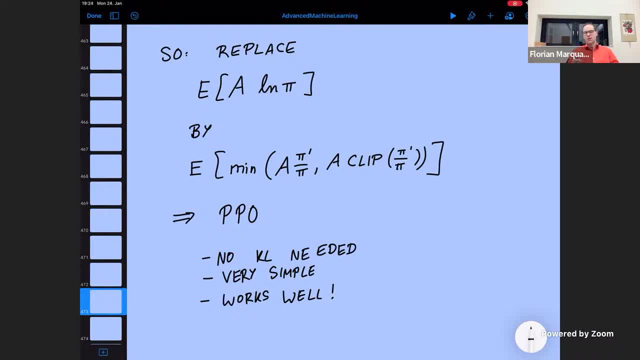 imagine the actions are discrete. but if we do so, this is only one direction when we safely say for. But if you have a control problem, like for a robot or for a qubit, then often you want to have continuous actions. So it's interesting to see how that works. 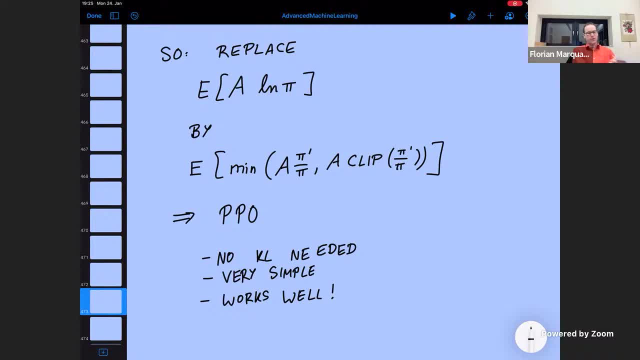 And then we will say something about model-based reinforcement learning. Everything we have described so far goes under the heading of model-free reinforcement learning. So the environment is like a black box. You don't need to know explicitly what goes on in the environment. 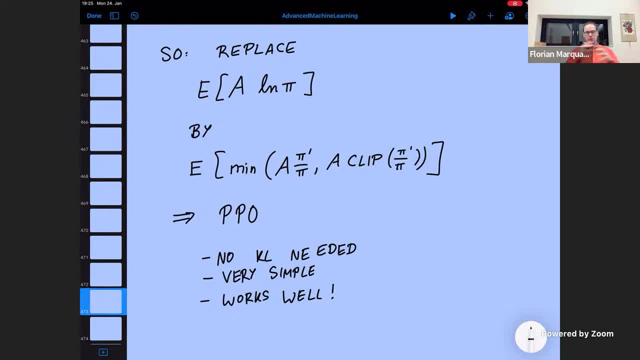 You are sampling everything And from then on you improve your policy somehow. In model-based reinforcement learning, you imagine that you do have explicitly on your computer a model of the environment, either a stochastic model or maybe even a differentiable continuous model. 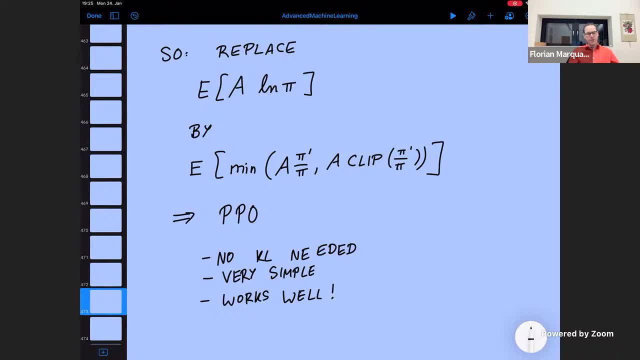 And then again you can ask the question: how do I proceed? And of course you can do a little bit of different things. You could sometimes take gradients through the whole model. That can be good. Or else you can do what is called planning.